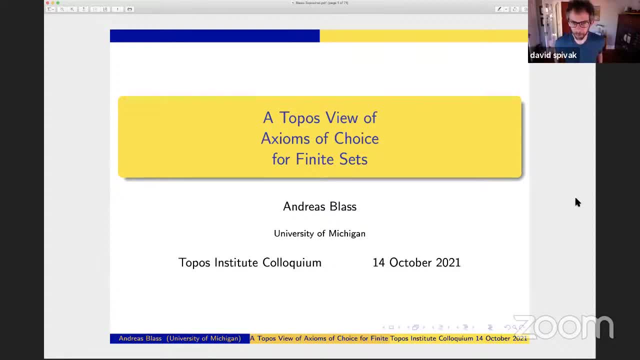 Okay, well, let's get started. So for people who are just joining, if you have clarification questions, ask at any time. It's even urgent to ask them if you need to understand something better And otherwise, feel free to also interrupt if you have other questions. 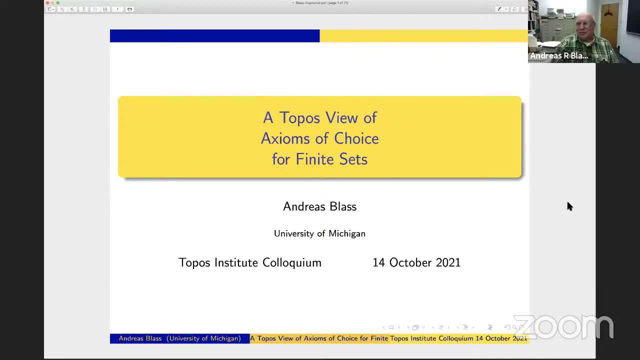 I mentioned that I'm unlikely to be paying much attention to chat, So if questions come up in the chat, somebody alert me audibly. Great will do So, great. So thanks everyone for coming Today. we are delighted to have Andreas Blass, a frequent contributor to our colloquium here and then on the other side, but finally talking to us about a topos view of axioms of choice for finite sets. So take it away, Andreas. 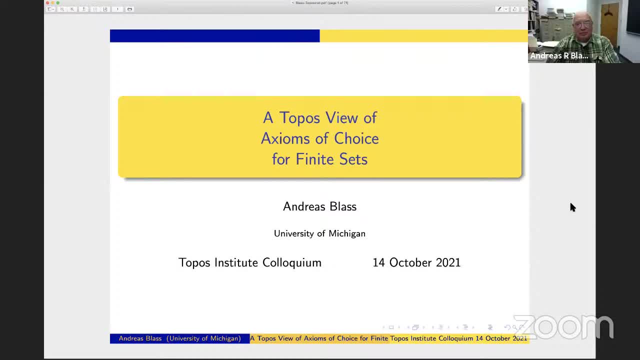 Okay, thank you. Okay, so I want to talk about axioms of choice for finite sets, And the first thing I better clarify is: the axiom of choice says: given a family of inhabited sets, there is a function that chooses one element from each. 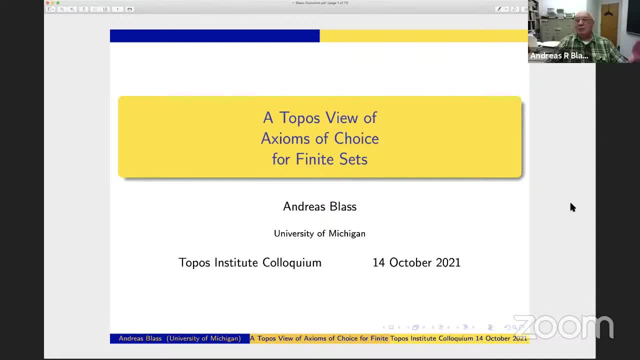 There are the index set of the family. there are the individual sets in the family. Finite sets here refers to the individual sets in the family. Choosing from a finite family of sets is something that can be done in some L Frankel set theory without any use of the axiom of choice. 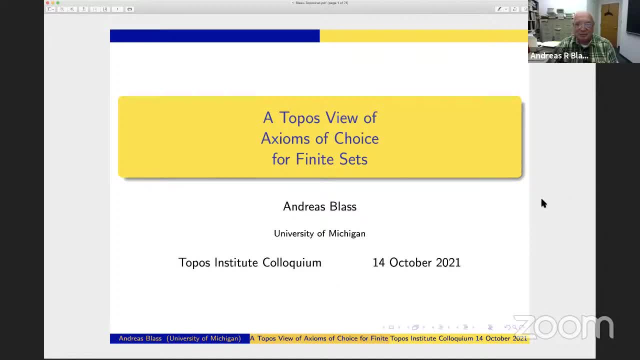 Finitely many choices don't require the axiom of choice For the sake of constructivists. if the index set is K-finite with decidable equality, then choice functions automatically exist. So I'm going to be talking about axioms that say, given a in general infinite family of finite sets, under what circumstances can we expect a choice function? So I'm going to be talking about axioms that say, given a in general infinite family of finite sets, under what circumstances can we expect a choice function? So I'm going to be talking about axioms that say, given a in general infinite family of finite sets, under what circumstances can we expect a choice function? 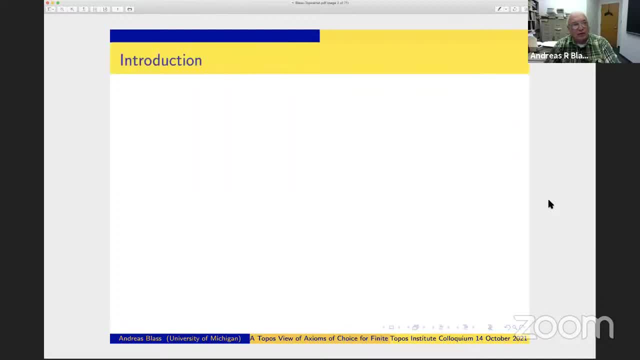 And as far as I know, the study of this sort of thing began with a result of Tarski which he never published. I think it dates from sometime in the late 1920s, but I'm not actually sure about that. 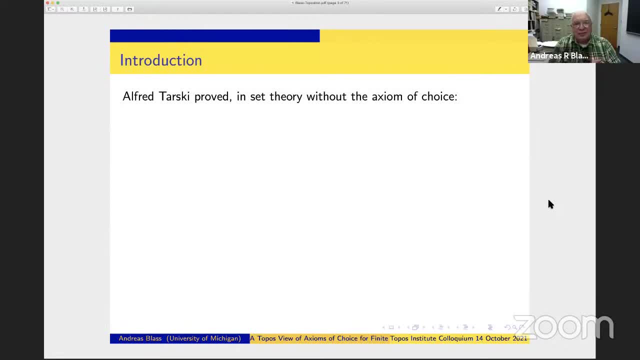 So he proved, without any use of the axiom of choice, that if you assume that all families of two element sets have choice functions, then you can prove the same for every family of four element sets. Now I should point out that the converse of this is really easy. 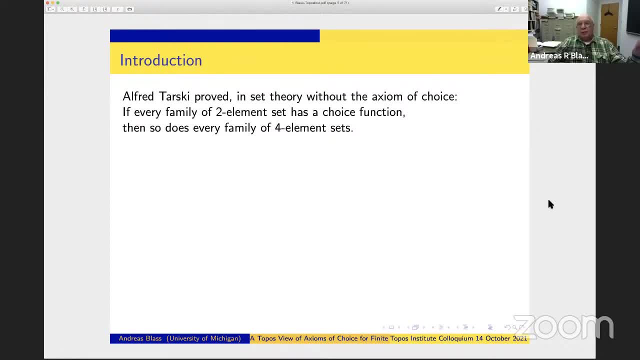 because if I know how to choose from four element sets and you give me a bunch of two element sets, I make each of them into a four element set by taking its Cartesian product with some fixed two element set, say 0,, 1.. 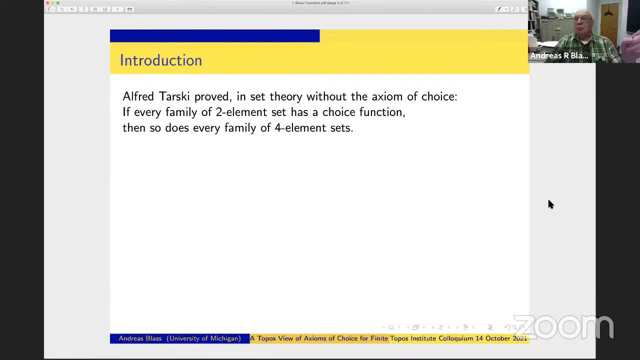 Now I have a family of four element sets. Let's pick an element from each of those and then just take the first component in that Cartesian product. So in general, if I can choose from families of sets of some cardinality, then I can do the same for any divisor of that cardinality. 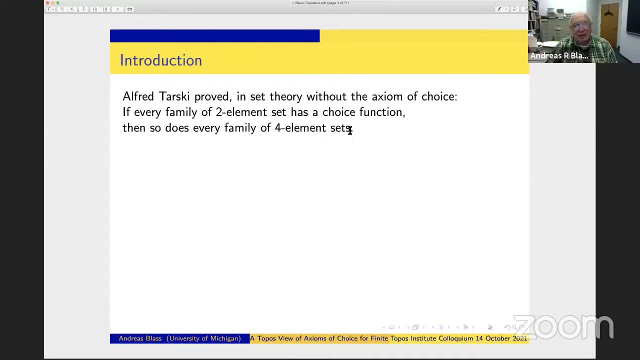 So not just from four to two, but divide by whatever number you like, But this direction, the direction that Tarski proved, is non-trivial. Excuse me just a minute I need to. I neglected to tell my phone not to interrupt me. 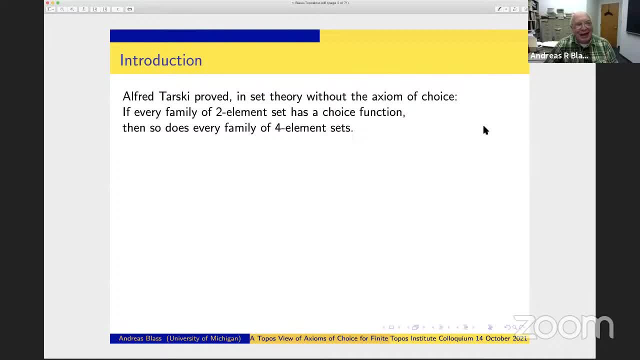 You can interrupt me, but the phone shouldn't. So let me indicate, since a colloquium should have at least one proof, and I might as well get it over with right away. So let me indicate how Tarski's proof goes. 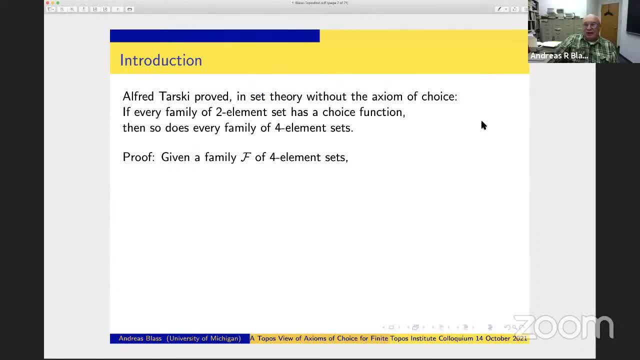 So we're given a family of four element sets. We want to choose an element from each. There's no loss of generality in assuming that those sets, those four element sets, are pairwise disjoint, because I can tag them with indices and so on. 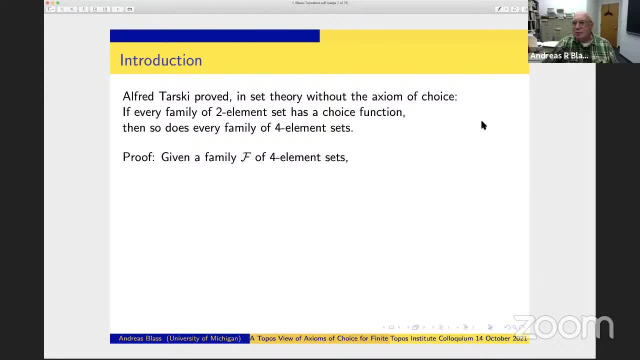 I don't think I'm actually going to use that assumption, but I'm going to wave my hands and say this set, that set and that set, without going that set and that set and like that. So, given a family of four element sets, here's what I'm going to do. 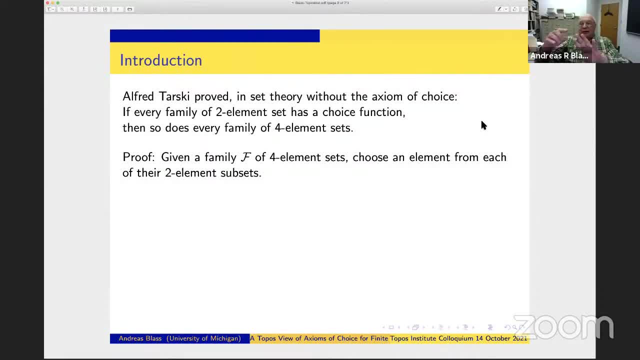 In each four element set. I'm going to have a set of four elements. I'm going to have a set of four elements In each four element set. choose from each of the six two-element subsets one of its elements. I can do that by assumption. 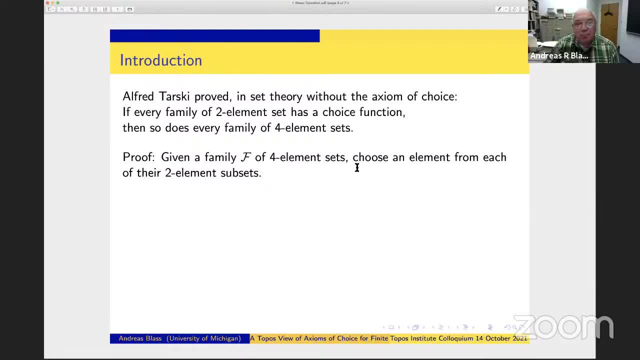 I'm choosing from a bunch of two-element sets. Okay, choose an element. So from each pair within one of these four element sets. I've made a choice. Now let's look at what happens inside one of these four element sets. 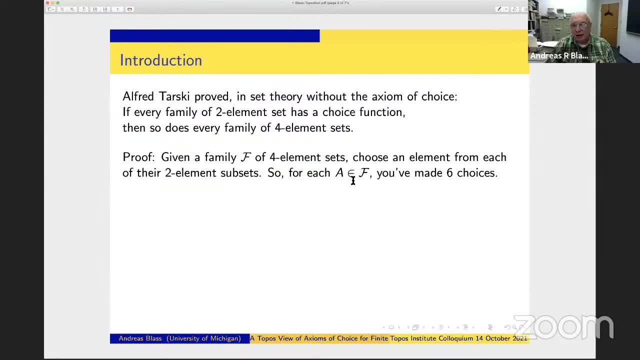 I've made six choices And I even wrote that on the slide. You made six choices, So the four elements in the set were not all chosen equally often because, by great good fortune, four does not divide six. So consider those elements in the four element set that were chosen most often. 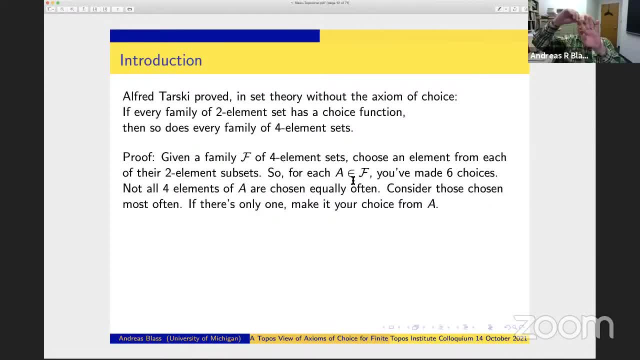 There might be just one of them. That can happen. You can have one element that was chosen from all three of the pairs that contain it and then each of the other elements was chosen only once. If there's a unique element chosen, most often that picks out that one element from your four element set. 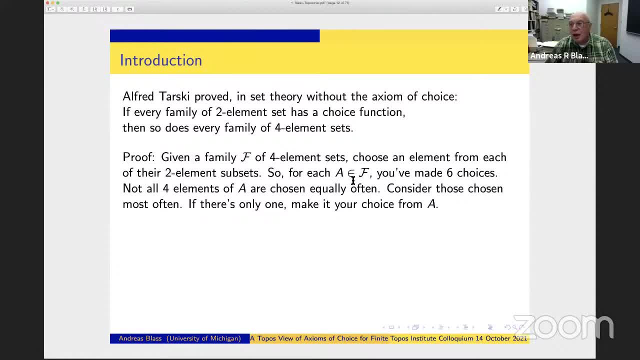 So that's your choice from that four element set. Another easy case is a three-way tie: Three chosen equally. often That can happen. also, Three elements can be chosen twice each and the remaining element not chosen at all. Well, in that case, take that remaining element. 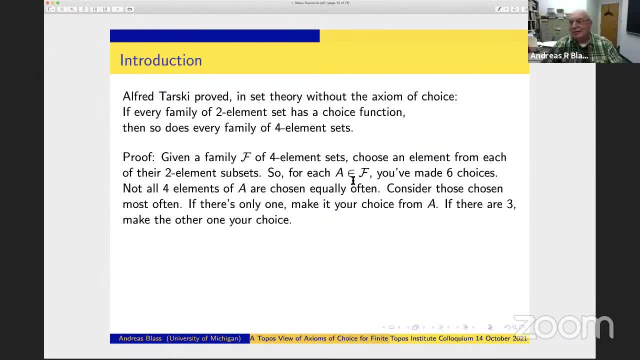 Take the loser. If there's a three-way tie for winner, take the loser And let that be your chosen element from that four element set. The last option is that there's a two-way tie, which also can happen. You could have two elements that were chosen twice each and the other two elements were chosen once each. 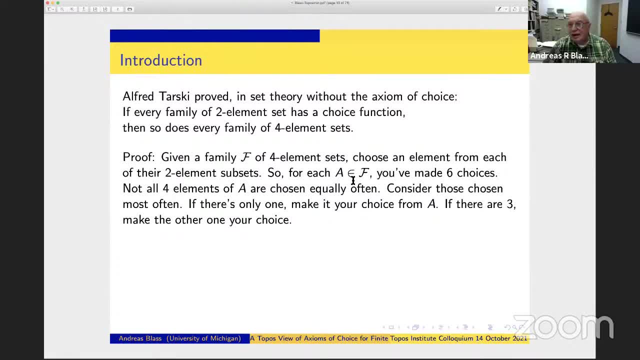 In that case, take the two winners. That's one of the two element sets from which you chose an element way back at the beginning, So you just take the one you chose. So in all cases, however, the distribution of choices works within any one four element set. one of those four elements is singled out, and that's how you get your choice function. 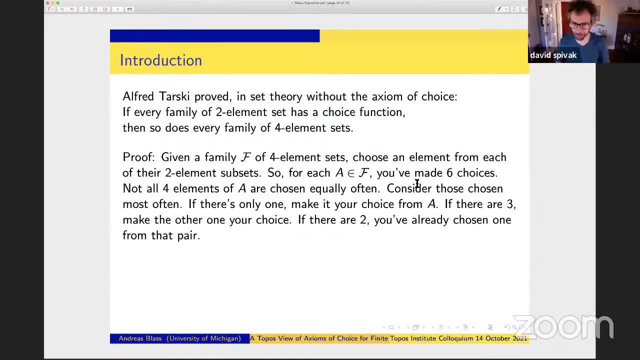 Andreas, can I ask a question? It's not quite clarification, but another strategy that I just want to understand why it doesn't work is: I take my family F and I replace it with a family 2F. It has two Fs. 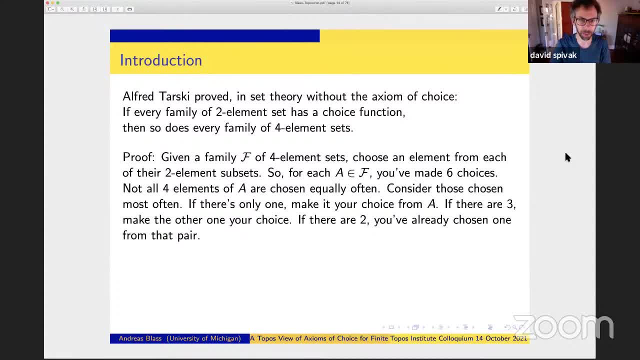 It has two F-many elements and each one is one of the original. So I take my four element sets and I think of them all as products of two times two, And now I have twice as a big family of two element sets and I just choose from each of them using my choice function, and then I pair. 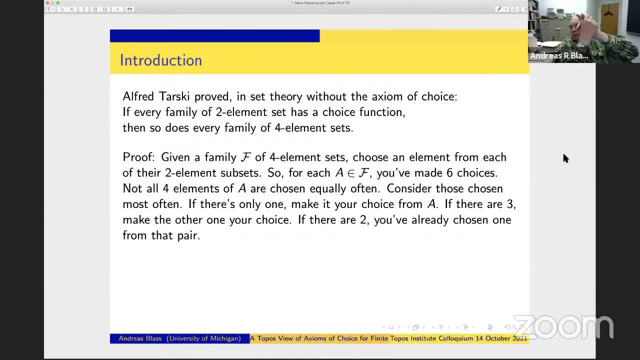 Each of the four element sets is sort of tearing apart into a couple pairs. Yeah, And then choose from those. That's right, Okay. So the first difficulty is you need to choose how to tear it apart. There are several ways to tear a four element set apart into two pairs. 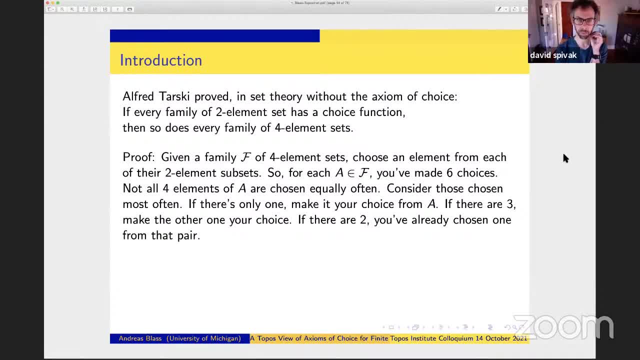 Mm-hmm, You can take any two elements and the complementary two elements. So there's some choice involved in that, which in fact we'll see again in a couple slides. And so if I have a proof that there are four element sets, isn't that an isomorphism to the number of four? 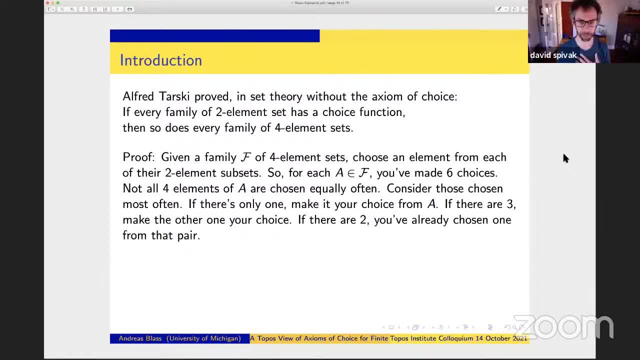 Pardon, If I have a proof that they are all four element sets, Isn't that proof giving me an isomorphism to four? Sure, If you have explicit bijections between all of these sets and the number four, or 0,, 1, 2, 3, or 1,, 2, 3, 4, or however you want to identify the number four, 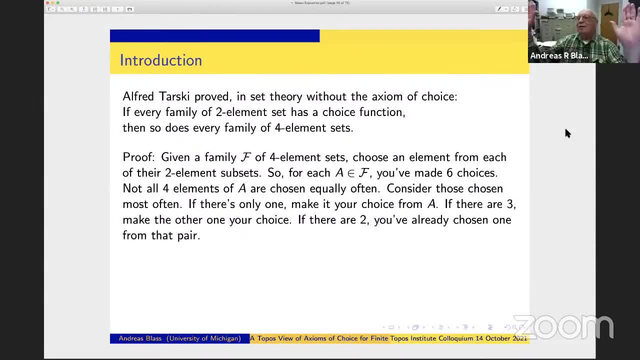 If you have those explicit bijections, then you're in great shape, because then I just take the bijection and apply it to one And that puts out the element right on top. Okay, great, Thank you. Thank you. That tells everything. 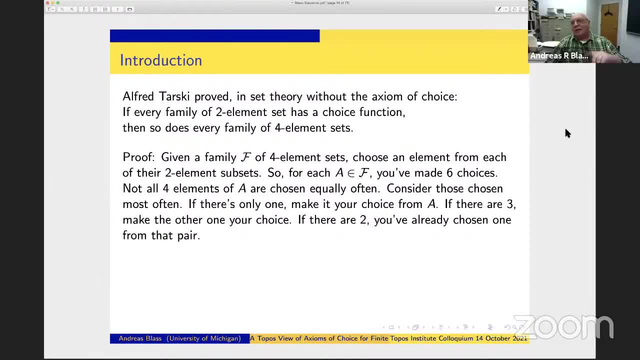 Yep, Thank you. Let me point out, even after solving everything, there's still another issue. Suppose I had each four element set torn into two element subsets, So now I have a twice as big family of two element sets. By assumption, I can choose an element from each. 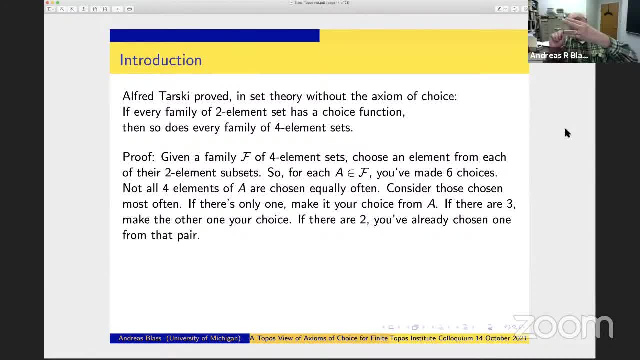 So what used to be a four element set is now two pairs and I've chosen one here and one there, But I need to know which of those two choice. Sorry, Yeah, I've chosen one here and one there, But I need to know which of those two chosen elements is the one that I want from my original four element set. 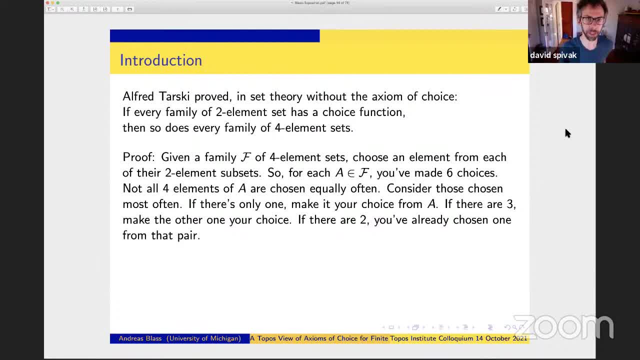 I was factoring it, not separating it. So there are a bunch of things going on here. Essentially, it's a quest. Let me get ahead of myself a bit. The real issue is: what kind of structure is available on these four element sets? 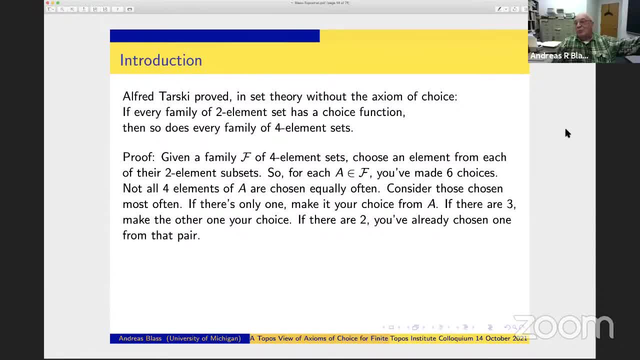 And a bijection to standard numeral four is sort of the most structure you could possibly hope for. Somewhat less than that would be a partition into two element subsets, Somewhat less than that would be. No, somewhat more than that would be an ordered partition: a two element set followed by another two element set. 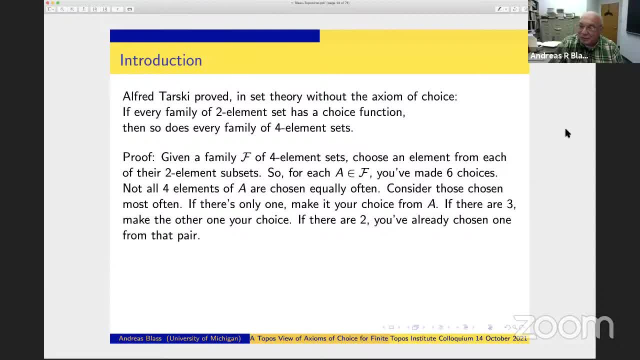 And for all of these things, one has to be rather careful to see what's actually. How much information is really there? Great, Thank you. As long as we're being careful, Let me, I've still got some room on the slide. 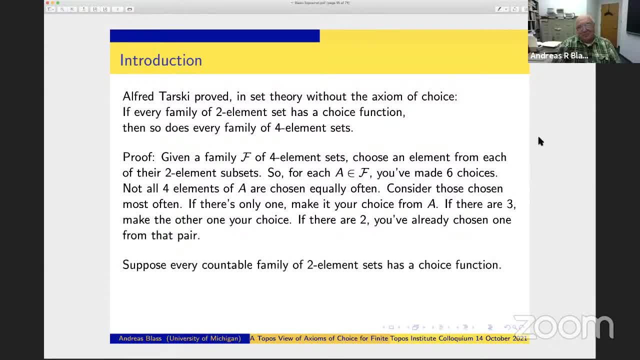 So there's some more carefulness coming. Suppose I change the hypothesis in Tarski's theorem just a little: Instead of every family of two element sets, I'm assuming for every countable family of two element sets, And I'd like to get the corresponding 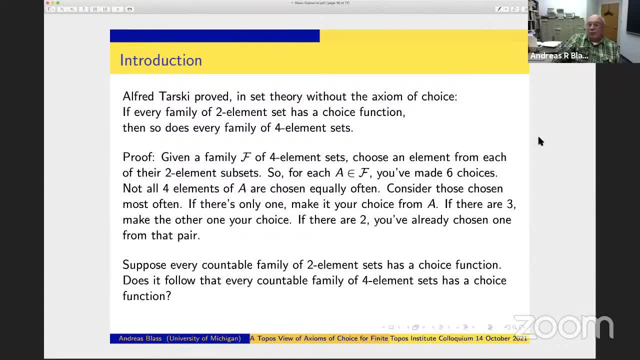 In conclusion, every countable family of four element sets has a choice function. I claim I haven't actually proved that, or Tarski hasn't actually proved that. That looks a little weird. I mean, let's look at the proof. 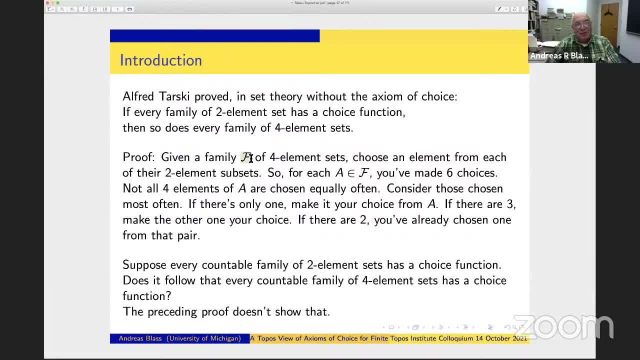 If you have, Suppose this family F is a countable family of four. element sets First one Countable family. I can assume it's actually enumerated First, one, second one, third one, I don't know. Now I want to choose. 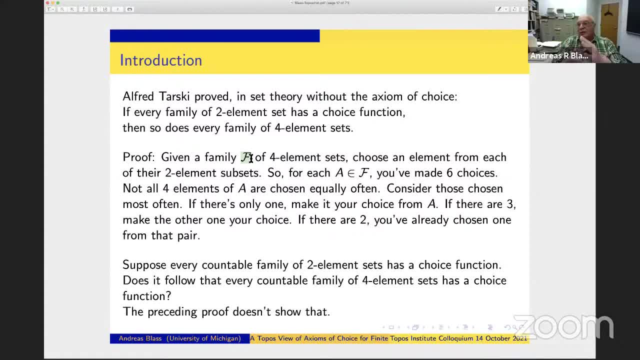 I want to take all the two element subsets and make choices from those. Each of the four element sets gives rise to six two element subsets, So the number of two element subsets that I need to choose from is countable times six, which is countable. 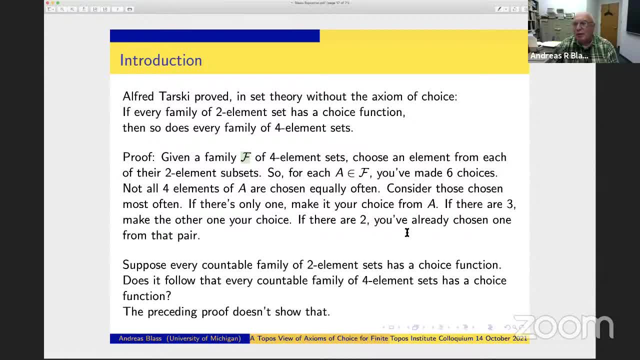 So countable family of two element sets? Well, no, Unfortunately, countably many six element sets do not necessarily add up to a countable set. How would you count it? Well, you count the six things in the first one, and then you count the six elements of the second, and then the six elements of the third, and so on. 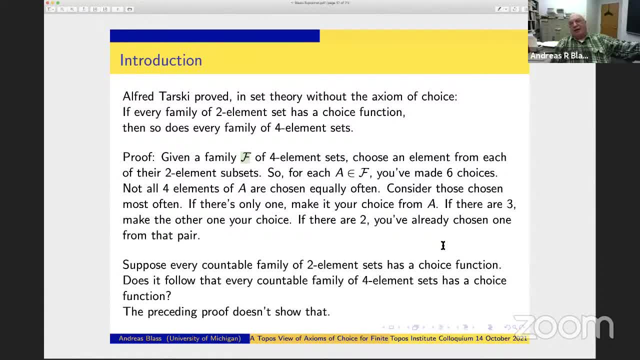 But in what order are you going to count? Well, those six elements. you can count them: One, two, three, four, five, six. Big deal, Yeah. but you have to choose an ordering in which to count them for each of those countably many sets. 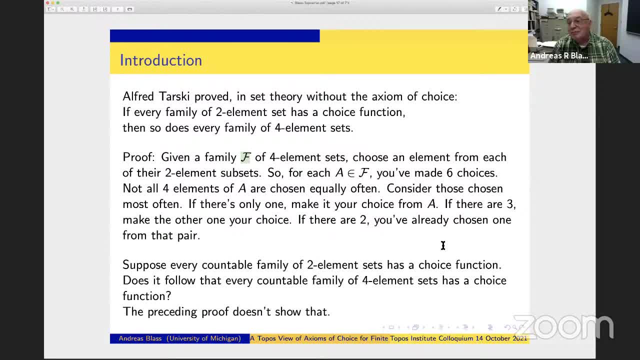 So you would be using another bit of axiom of choice there in order to say that you're dealing with only countably many two element sets. So Tarski, with this proof, did not actually prove the countably indexed version of the theorem. 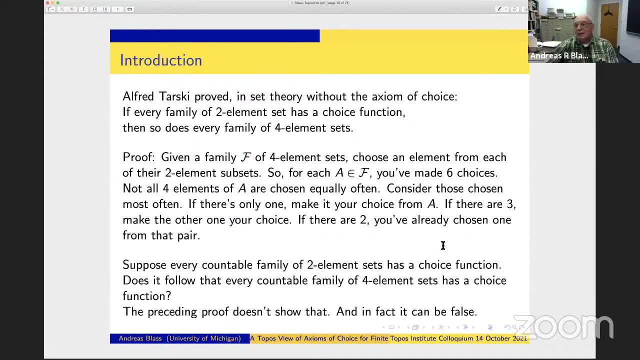 And that's a good thing. And that's a good thing because it's false, Not only not proved by Tarski's proof, it's not provable in Zermelo-Frankel set theory. Maybe I should say something about not provable. 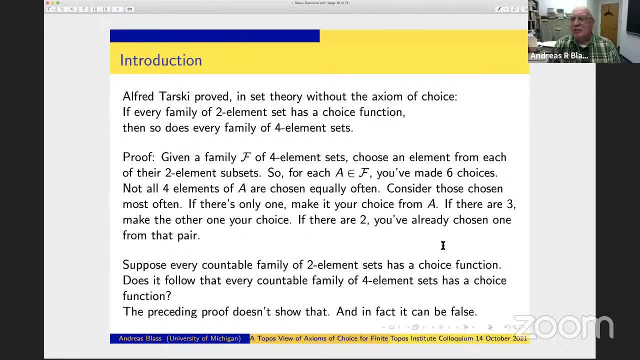 Oh, Zoom says participants can now see your application. I've been assuming you can see the slide all along. Are you seeing anything else? I'm not seeing anything else. Okay, Maybe Zoom is just slowly noticing that you're seeing my slide. 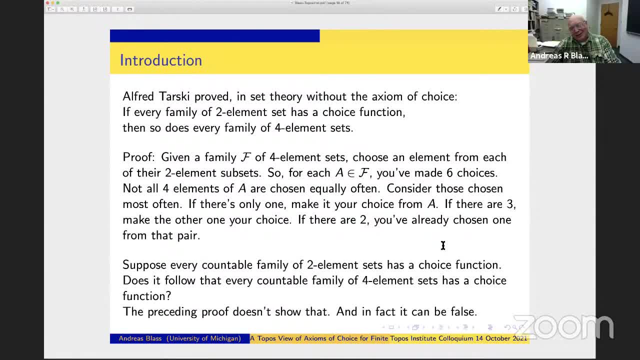 Okay. So how does one know that something like this can be false? Well, one constructs models of set theory in which it's true that every countable family of two element sets has a choice function And it's not true that every countable family of four element sets has a choice function. 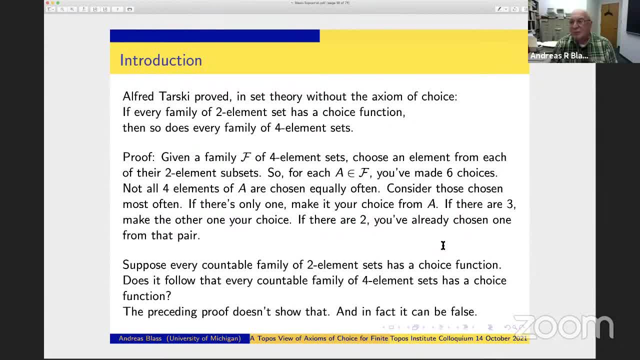 How does one construct models of set theory where weird stuff happens? Well, since the 1960s we've had this forcing technique, viewed at Cohen, which we used to get the independence of continuum hypothesis and the axiom of choice and so on. 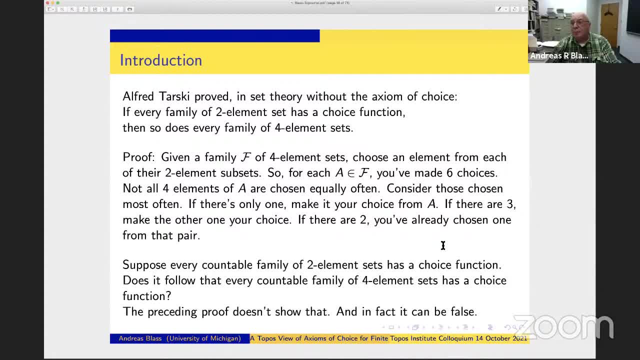 But I'm talking about Tarski in the 1920s. What would he have done? I'm not sure he actually checked that. it can be false, But the methods were available, Namely the method of permutation models. Strictly speaking, it doesn't apply to ZF. 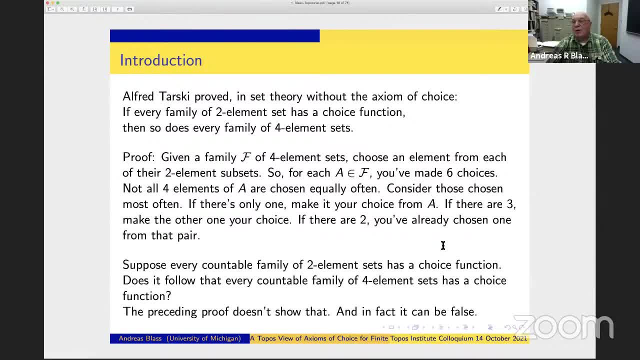 It applies to ZF modified to allow for atoms, Things that are not sets but can be elements of sets- A rather natural set theory. You know there's lots of stuff here, like my COVID mask and my pen and my nose and so on, that are not sets but can be elements of sets. 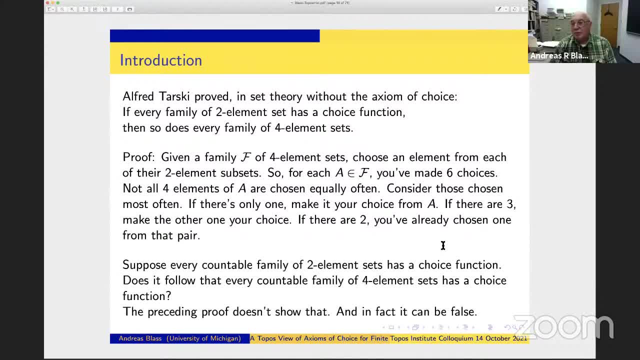 In that context it's much easier to get independence results And in fact Franco had already proved the independence of the axiom of choice under those circumstances back in 1922.. So the notion at the bottom of the slide here of something like this can be false. 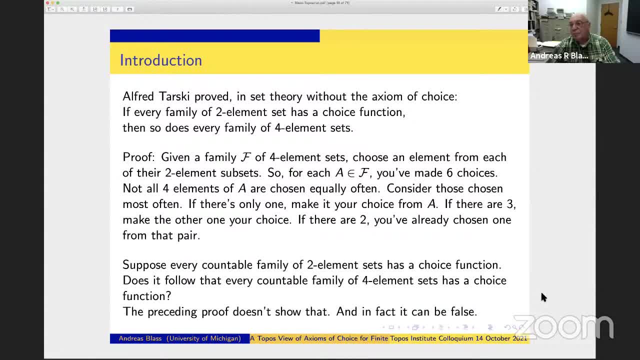 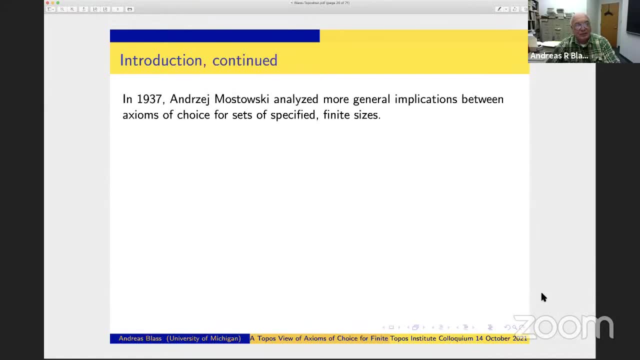 There were methods available. There were methods available to show that such things can be false. They may not have been well known yet, But they had been developed, in particular by Franco. Okay, The next bit of the story, Moving ahead to the 1930s. 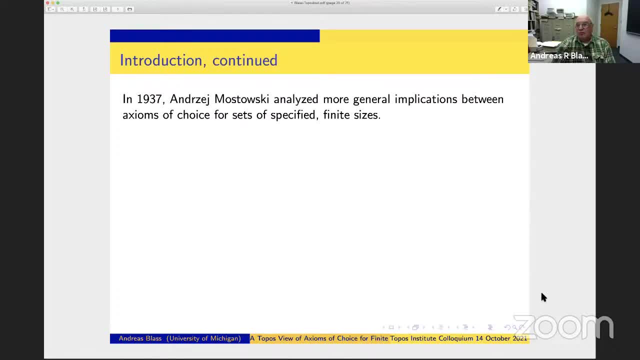 Mostovsky analyzed the situation in more generality: Implications between axiom of choice For sets of specified finite sizes. I might add that in this 1937 paper of Mostovsky he actually did present Tarski's theorem with Tarski's proof, with correct attribution. 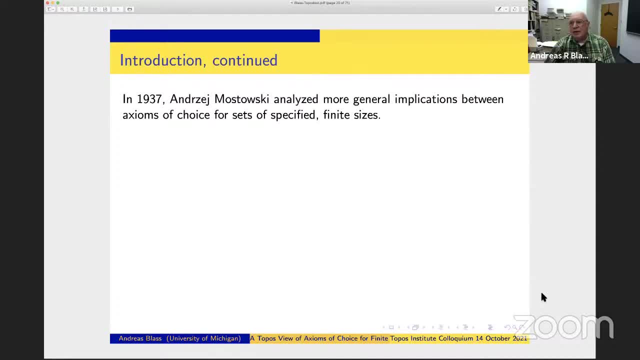 He says that this is a theorem of Tarski. He presented it in the fine print, And I really do mean fine print literally. I mean it's a paper in Fundamenta, And this result and the proof of Tarski's are printed in smaller types. 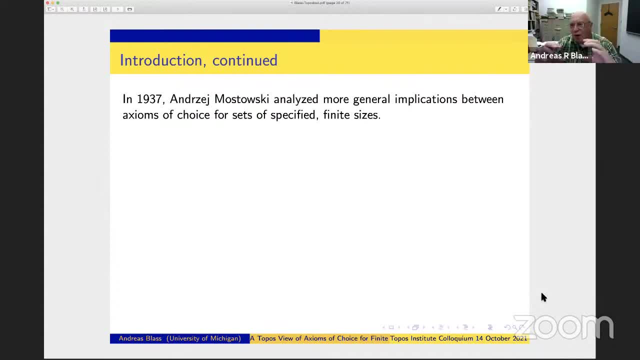 It's not a footnote. It's in the main text, But it's smaller than everything else in the paper. So this is sort of the fine print of Mostovsky's paper. So what did Mostovsky do? By the way, those of you who know about models with atoms that violate the axiom of choice probably know them as Franco-Mostovsky models. Sometimes Franco-Mostovsky-Specker models. This paper and some others around the same time are Mostovsky's contribution, essentially generalizing Franco's method to get a lot more independence results. So Mostovsky obtained some number theoretic and group theoretic conditions for provability. 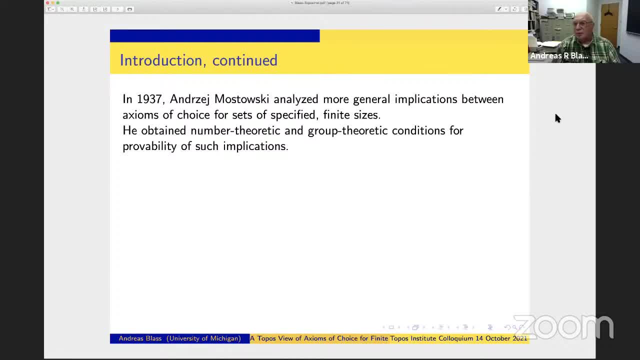 We've already seen that number theoretic things. at least some very simple number theory is relevant. in Tarski's proof, The fact that six isn't divisible by four was important- That we don't have a four-way tie between all the elements as to how often they get chosen. 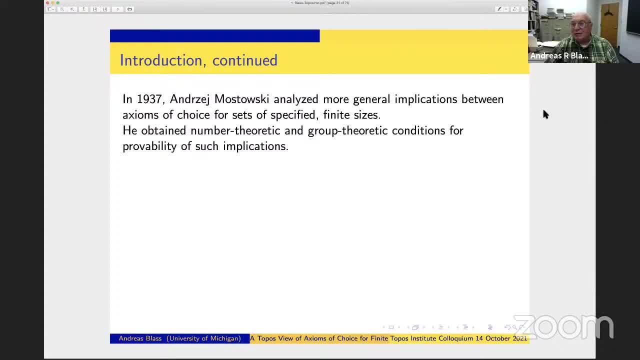 Group theory also shows up in the idea that, well, the amount of structure on these sets can matter, Like can I split them into pairs? Do I have any structure at all on them, And so on, And this can be described in terms of automorphism. 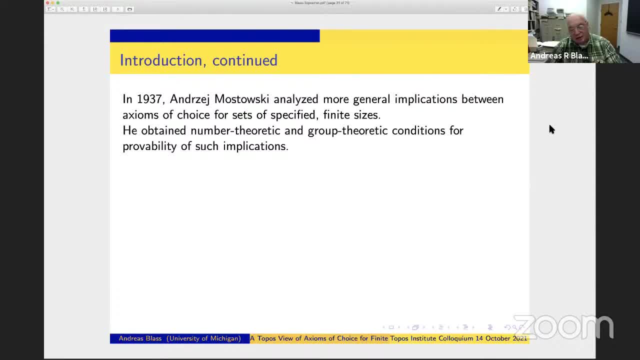 And so on, And also group theoretic ideas are involved in the Franco-Mostovsky method for building independence results. So it's not surprising that he got conditions of this sort. He had some necessary conditions And he had some sufficient conditions, But none of his. he didn't prove that any of his conditions were simultaneously necessary and sufficient. 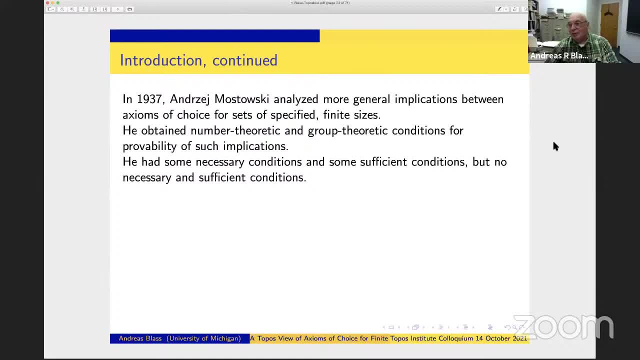 So he didn't get complete information about implications between these various choice from finite sets principles. Okay, So his conditions were enough to settle a lot of cases, but not quite all. The first question that was not settled- and he mentions this explicitly toward the end of the paper- is this: 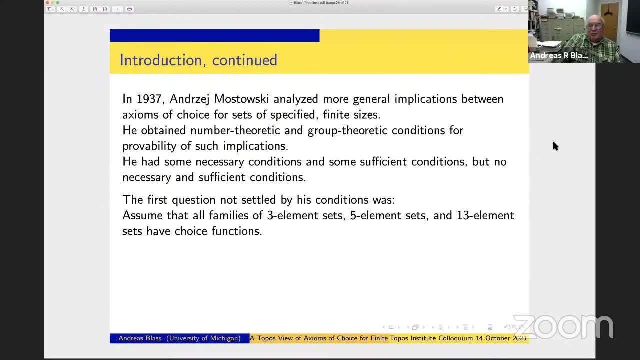 Assume that you have choice from families of three element sets, five element sets and 13 element sets. Before I finish stating the question, let me point something out. There is an ambiguity here which fortunately doesn't matter, but I should point out that it doesn't matter. 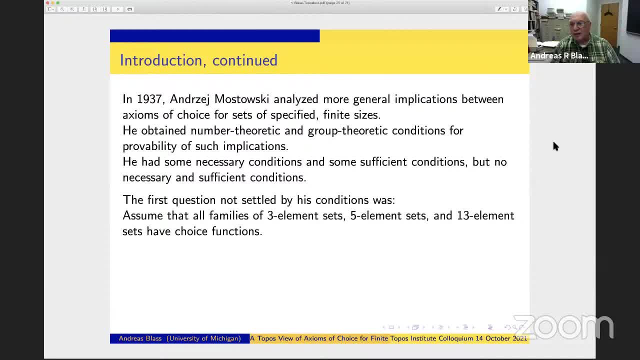 Is this three separate assumptions- choice from three element sets, choice from five element sets, choice from 13 element sets- or is it an assumption that you can choose from any family of sets whose sizes are among three, five and 13?? 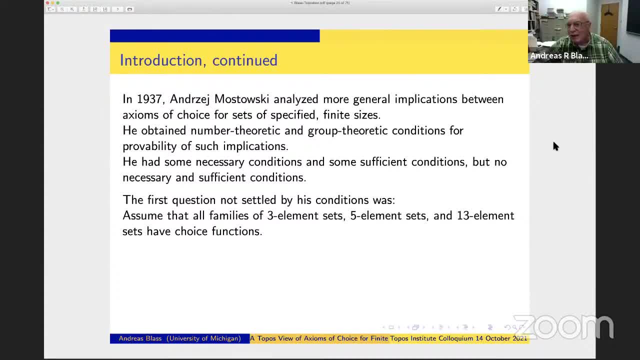 Even if they're all sort of mixed together in one family. And the answer is, it doesn't matter, Because if you had them all mixed together, you could take the subfamily of three element sets, the subfamily of five element sets, the subfamily of 13 element sets. 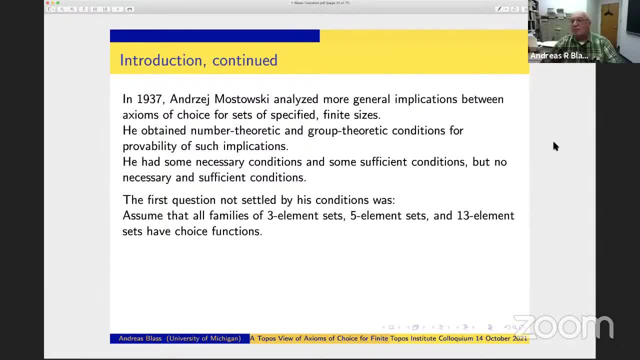 If you get choice functions for each of those subfamilies, you could just pick one choice function for each and glue them together to make a choice function for the original family. I emphasize: the word pick Sounds dangerously like axiom of choice, but I'm only making three choices. 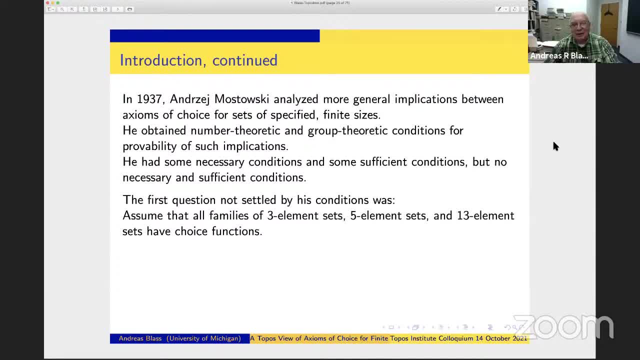 And three. thank goodness is finite. Okay, So it doesn't matter which side of the ambiguity you interpret this, as It's the same assumption in any case. The question is: does it follow that all families of 15 element sets have choice functions? 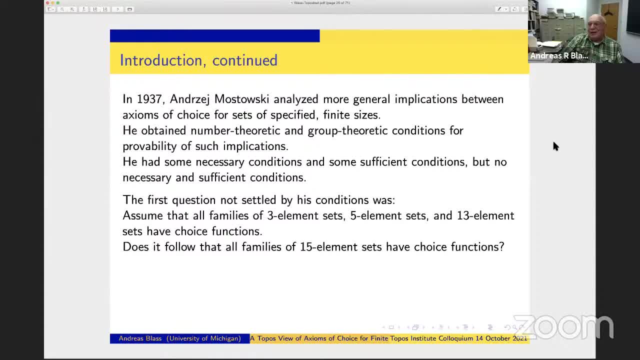 So this, it looks like a totally random question: Why three, five, 13,, 15?? But the answer is that, essentially, anything simpler than this was settled by Mastofsky's necessary conditions or Mastofsky's sufficient conditions. So this was the remaining open, well, the first remaining open problem. 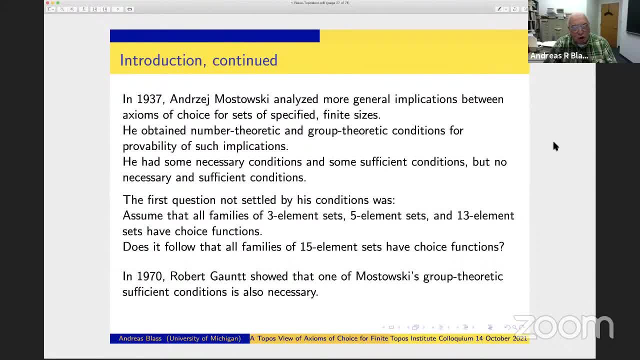 And all of this was settled by Robert Gaunt in 1970, assuming that one of Mastofsky's group theoretic sufficient conditions is also a necessary condition, And I'll put that condition- I think it's on the very next slide. 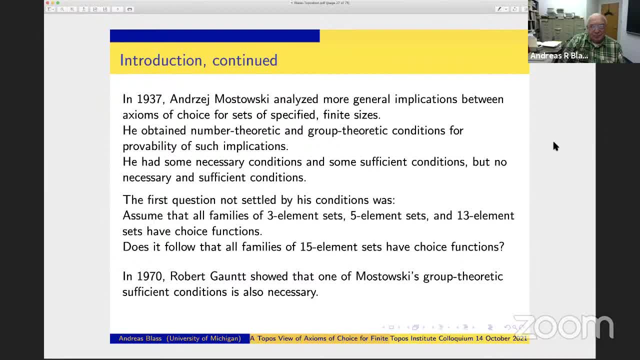 unless I inserted some intermediate proofs. In particular, choice from three element, five element and 13 element sets does not imply choice from 15 element sets. This publication record on this is somewhat sketchy, So following in the tradition of Tarski with his original result, 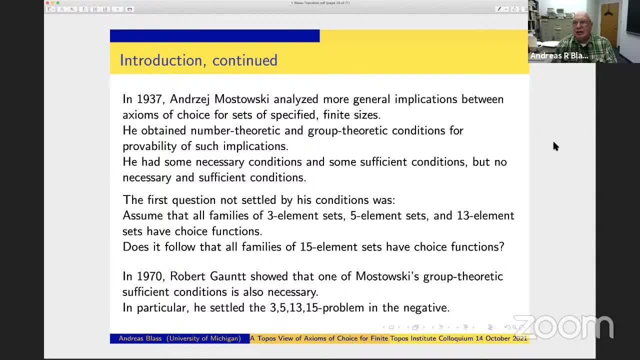 Gaunt wrote a PhD thesis dated 1969, in which he got a lot of results about these finite axioms of choice, but not the sort of final solution of Mastofsky's questions. That came a bit later, As I said here, 1970. 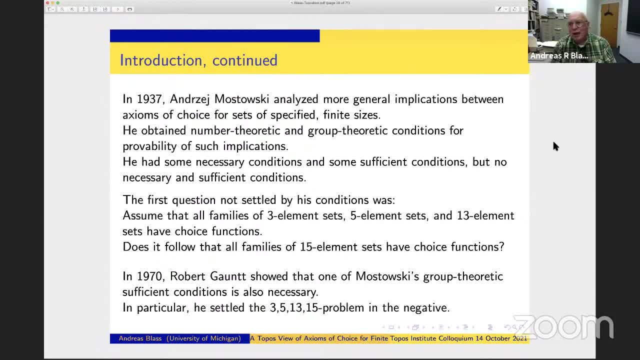 His thesis results were already announced in an abstract in the notices of the AMS in 1968.. The result I'm citing here was also announced in the notices of the AMS in an abstract in 1970.. As far as I know, Gaunt never published this. 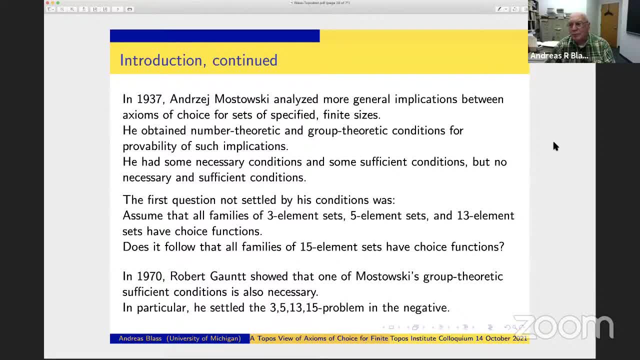 I think he wrote it up. I've heard references to it, His preprint- But I've never actually seen it. Fortunately, John Truss wrote in- I think 1973, a rather extensive paper in the Annals of Mathematical Logic. 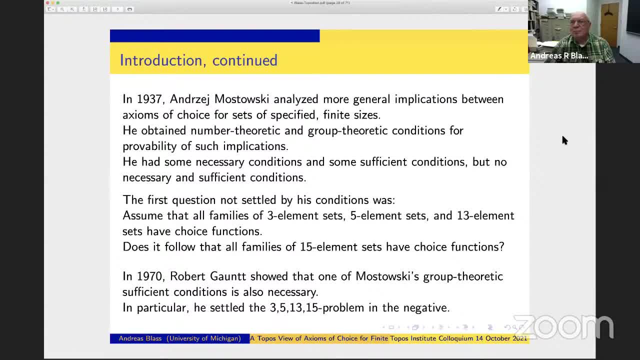 Oh, in those days it was Annals of Pure and Applied. No, Back then Annals of Mathematical Logic, Now Pure and Applied Logic, An extensive paper giving Gaunt's results and some considerable extensions of them also. So these results are available. 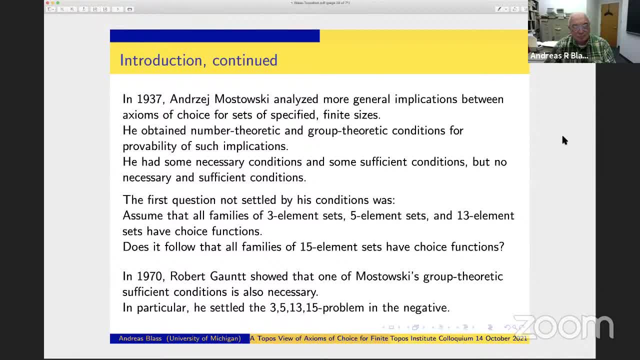 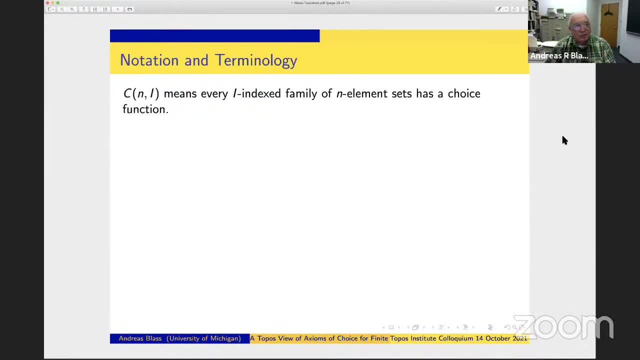 but Gaunt himself never published them. Okay, What did I do next? Oh, notation Terminology Good, So I can abbreviate stuff. Notation choice from n element sets indexed by i: Every i-indexed family of n element sets. 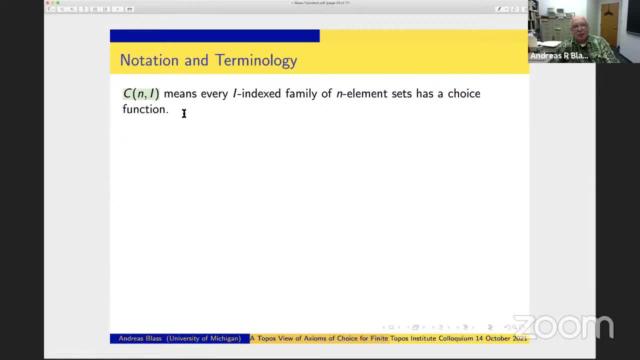 has a choice function And, as you saw in the Mostovsky's 3-5-13-15 problem, we'll sometimes have hypotheses that say choice like this for several n's at a time. So I have an abbreviation for that. If I have a set z. 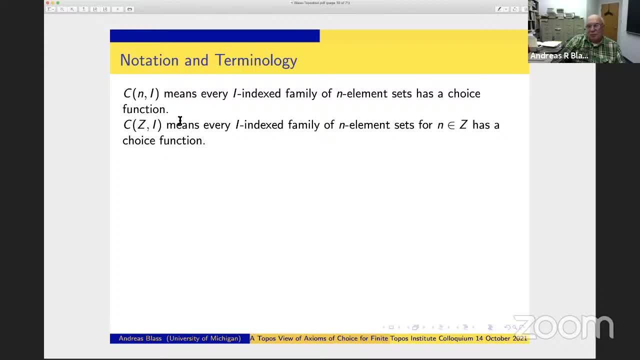 then putting that in place of n just means same choice principle for any n in z. Okay, So Tarski's theorem, for instance, says that if you have for all i, c2i, in other words choice from pairs, no matter what the index set is, 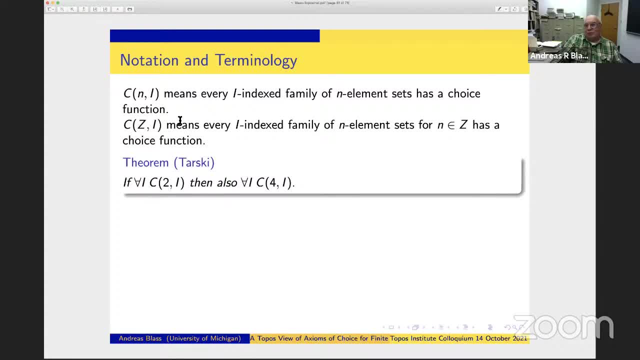 then you also have for all index sets choice from four element sets. The result that I said earlier is false. I said it's false if you only work with countable things. It's even falser if you make this stronger statement that for each individual index set. 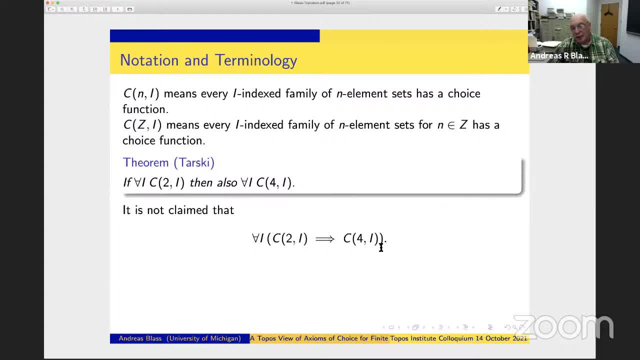 choice from i-indexed many pairs implies choice from i-indexed many four element sets, So this is not part of Tarski's claim. It is, however, true, and I think this is also due to Tarski, but I'm not sure. 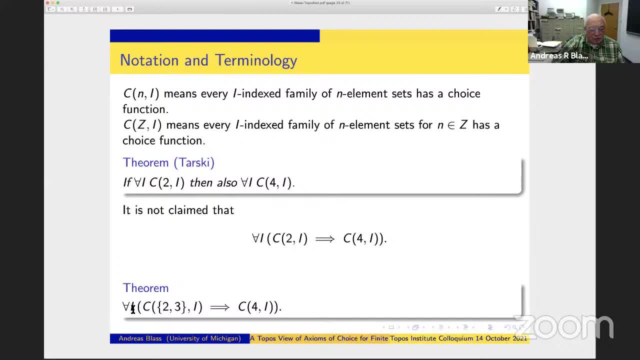 that if you assume for any particular index set, choice from i-indexed pairs and i-indexed triples, then you get choice from i-indexed four element sets. Okay, And I think I actually gave a proof of that. Oh no, 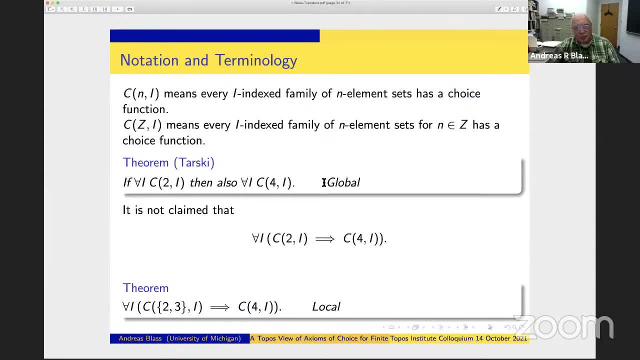 Before I go to proofs, insert some terminology here. I refer to this last version where you do it for each index set individually, Get the result for this index set from the hypotheses for the same index set. This I call the local implication between those choice axioms. 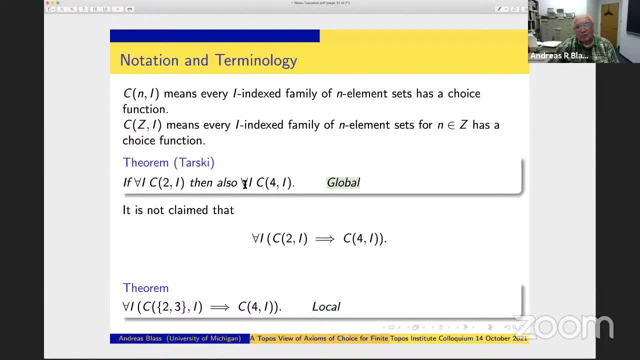 The sort of thing up above where you get the result for any index set but assume the hypotheses for possibly different index sets. That I'm calling global because you're making an assumption about all the index sets to get the result even for one index set. 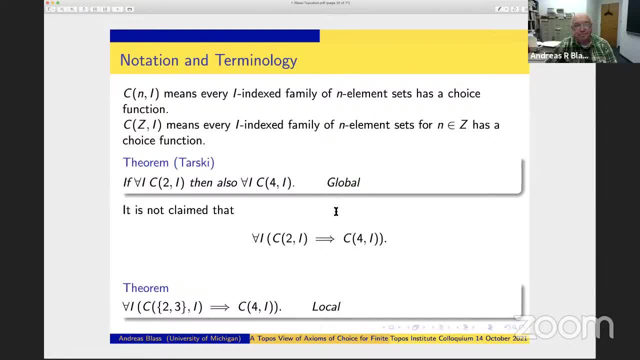 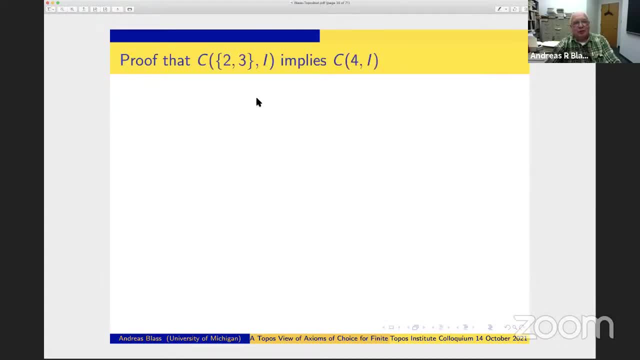 So the local version is the stronger of the two. Okay, Now I think I have a proof. Yeah, So this is the proof of the local implication. if you can choose from i-indexed pairs and triples, then also quadruples, And the good thing about this proof is it's nice and short. 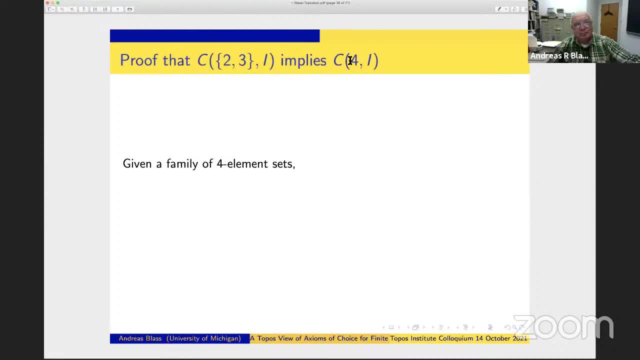 You can tell, because it begins in the middle of the slide and Beamer makes them symmetric. So if there's that much space above, there's going to be similarly much space below and not much proof. So, given a family of four element sets, 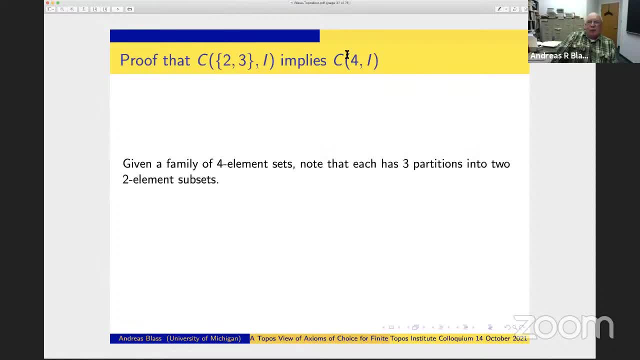 whatever the index set is, each one can be partitioned into two two-element sets. This is what David was going to do, but it can be done in three ways. Right, This way, this way, and something I don't want to try with my hand. 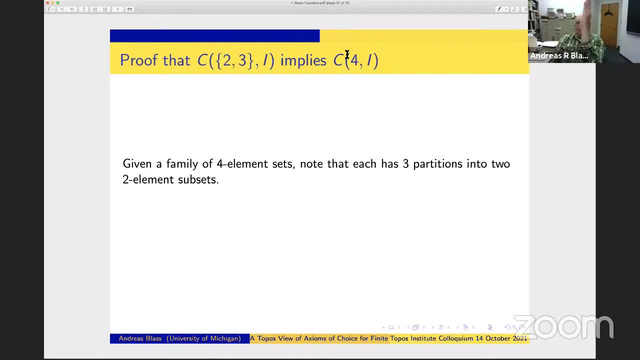 Line the four elements up in a square and you can cut it this way, cut it this way or use the two diagonals, But of course you can't really line them up in a square because that picks a linear ordering of the elements. 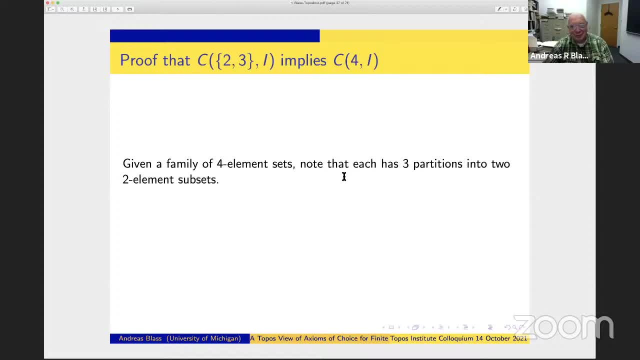 So this is your picture. It's how you see that there are three partitions, But we can choose from triples as part of the assumption, So we choose one such partition for each of the given sets. Now, each of these, in each set, we have the chosen partition. 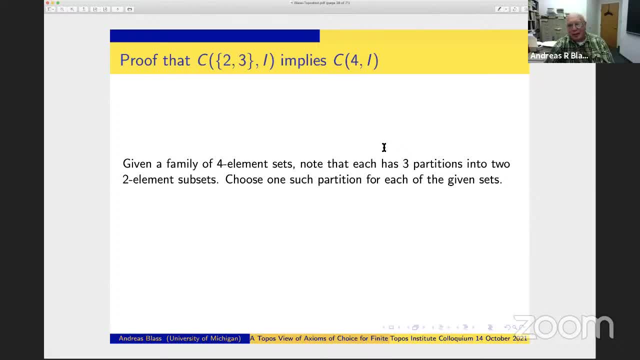 It has two pieces. We can choose from pairs. So choose one of the two pieces of that partition. Now we've got one piece, a two-element subset- We can choose from pairs. it says So choose an element from the chosen piece. 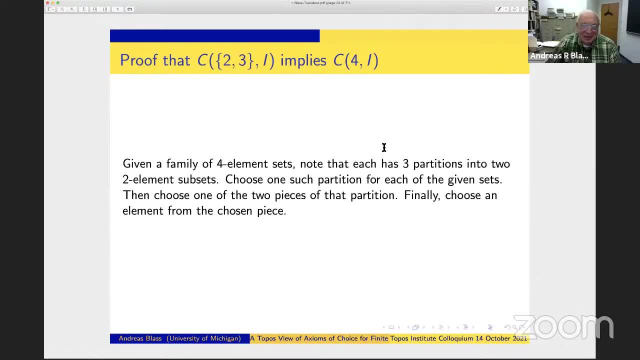 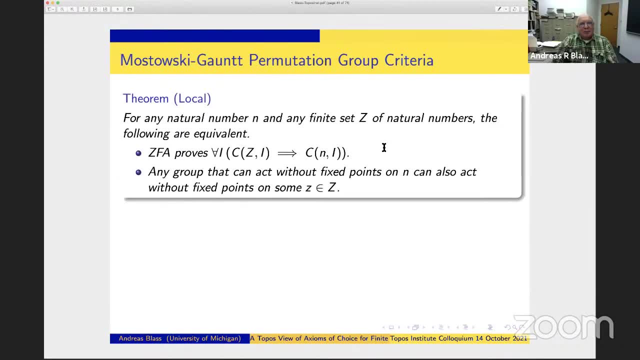 of the chosen partition. That's the end of the proof. Just as well, because I don't want to run out of time. So I promised you the Moustafsky-Gantt permutation group criteria. So these are. when can you prove? 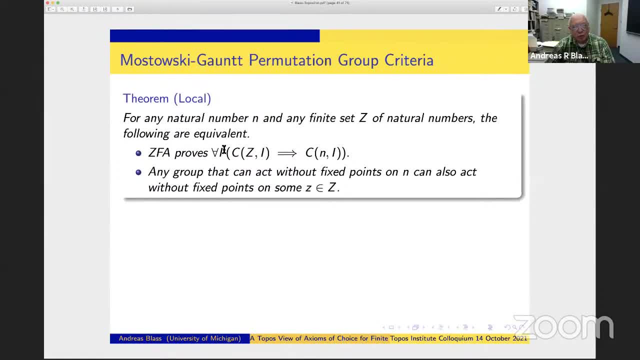 oops, not that. yet This is the local theorem, So I'm trying to prove a local implication for each index set separately. Choice from sets of cardinality in Z implies choice from sets of cardinality N And the criterion is in group. theoretic terms. 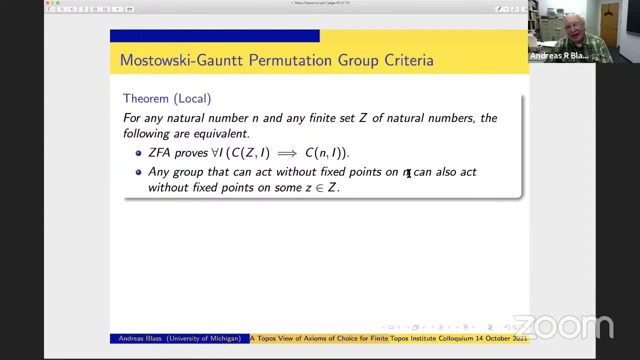 any group that can act without fixed points on N- meaning on an N-element set- can also act without fixed points on some Z. A fixed point is just a point that's fixed by all the elements of the group action. I should be a little bit careful here. 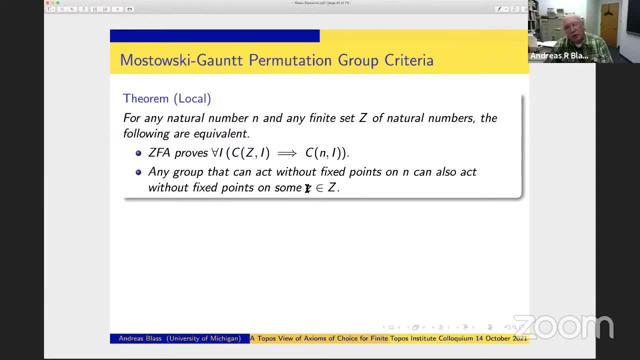 That criterion, the group theoretic criterion, shows up as shows up in Moustafsky's work, shows up especially in Gantt's work. They present it not specifically as a criterion for this local implication, They have it as a criterion for. 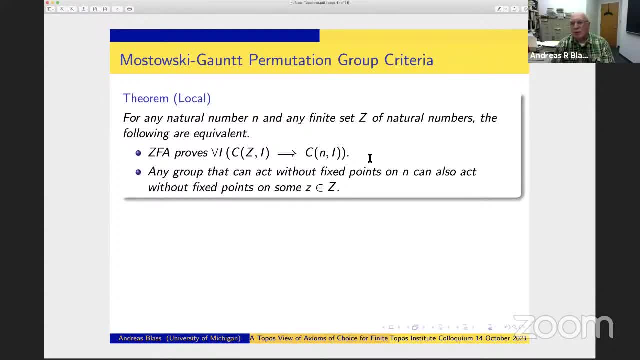 say the implication when i is countably infinite, And I think Truss has it for, more generally, when i is any well-ordered set, and so on. Andrea, someone in the chat is asking what ZFA is. Oh, yes. 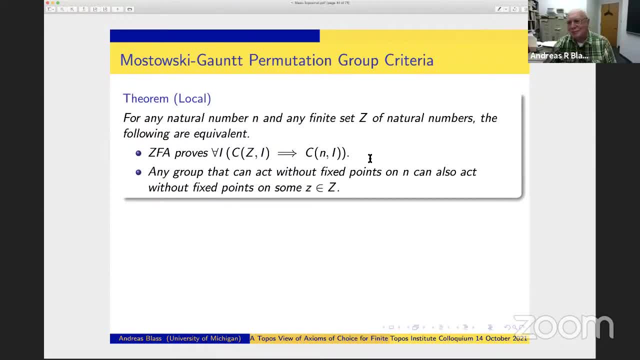 good point. ZFA is ZF with an extra A on the end for atoms, So it's ZF modified to allow for atoms. In fact, I should make an additional comment about that now that it's out in the open. I said a moment ago that. 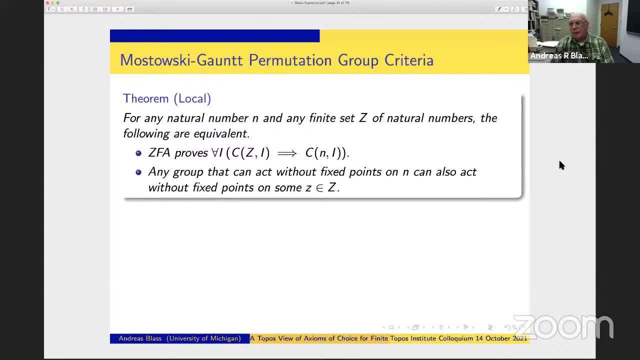 although we now have forcing methods to prove independence results, back in the days of Tarski and Moustafsky, all that was available were these Franco-Moustafsky methods that involved required actually having atoms available, which is why they do this work in ZFA. 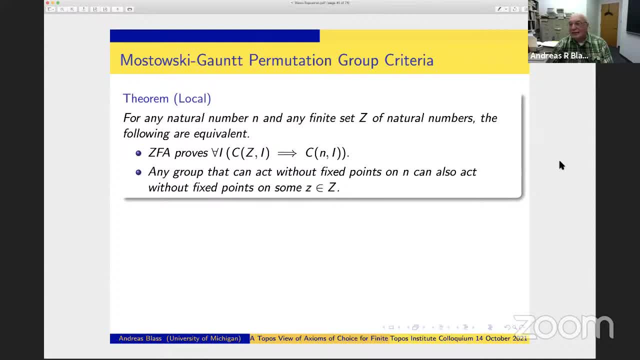 We're talking now also about Gaunt's results 1970.. Forcing was available and I think Gaunt did use forcing, But in fact for the sorts of implications that I'm talking about here, it doesn't matter. it turns out. 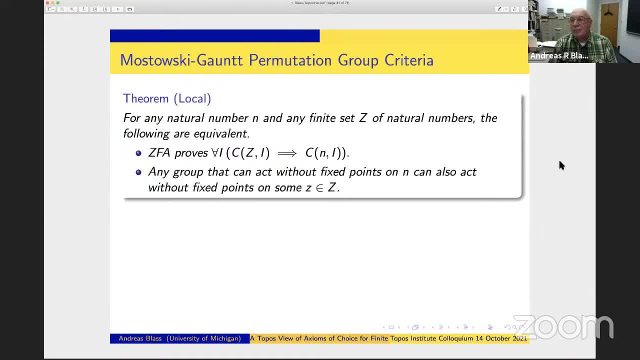 in the end that whatever you can do with the easier methods of Franco and Moustafsky could also be done with forcing to get models that don't use atoms. This is not entirely trivial. No, this is not even anywhere near trivial. 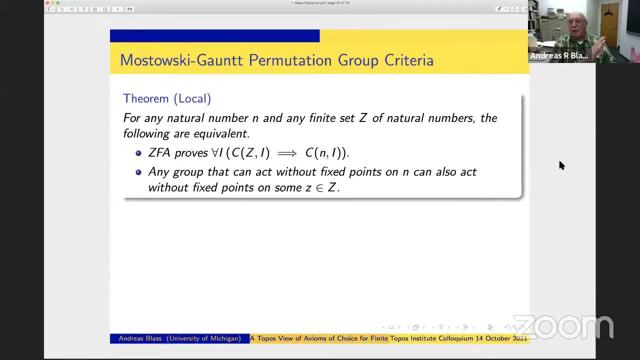 There are transfer results from models of set theory with atoms to models of set theory of the standard sort- pure sets, no atoms, And the transfer, the original transfer result, is a theorem of Yech and Sohor which I don't think will quite cover these implications. 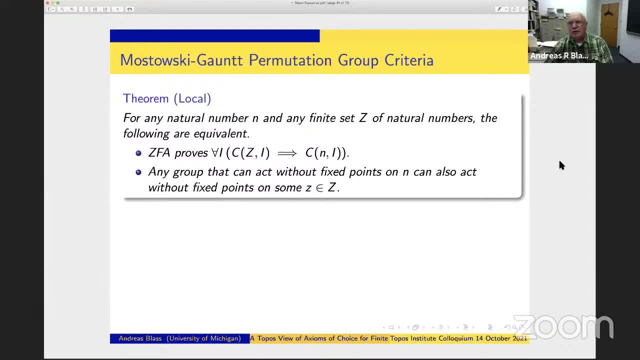 But David Pincus in his PhD thesis- which I think is around 1969, established more general transfer results which do cover these things. So in fact I could have left off the A and avoided the question, but since the question actually leads to interesting information, 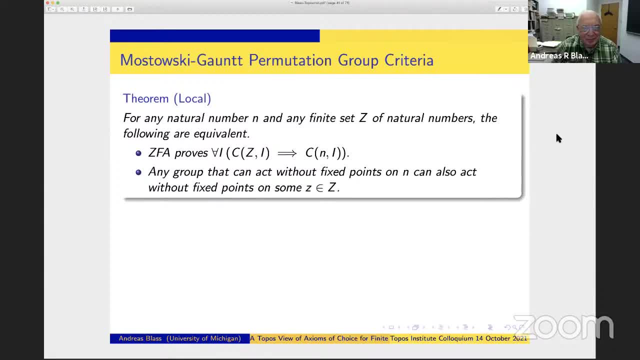 I'm kind of glad I left the A in there. I should add that the actual proofs that I end up doing whenever I do any of this stuff- I just use the atoms and then rely on Pincus's transfer theorems. Okay. 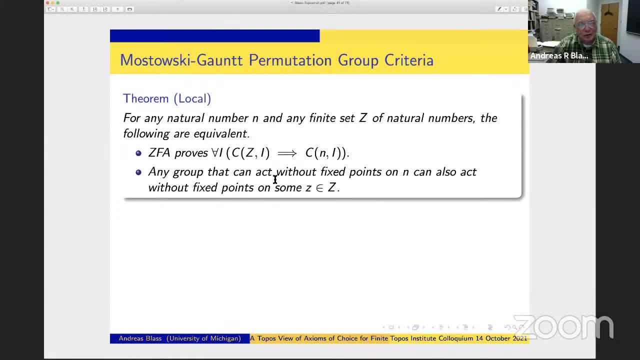 It may very well be that the first place where literally this theorem is proved is in a paper of mine on interaction between set theory and category theory from 1983. But the ideas are the same as in the work of Mostovsky and Gaunt. 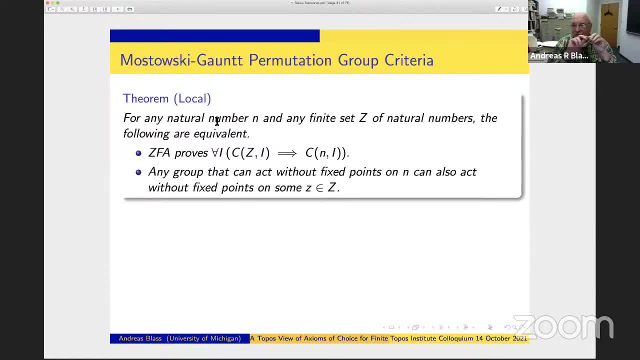 It's just specializing it down to the specific local case. rather than countable sets, well-ordered sets, whatever, There is a similar result for the global case. So again, N and Z are arbitrary. Z is a finite set of natural numbers. 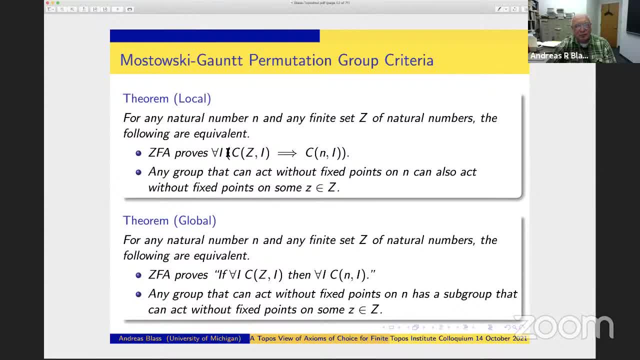 Finite is important to avoid that ambiguity I talked about earlier. So the first bullet item here is the global implication. If choice holds from Z element sets, no matter how indexed, then it also holds for N element sets, no matter how indexed. So this is a weaker statement. 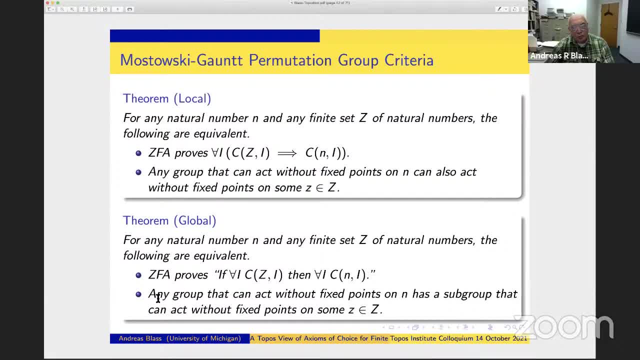 than the local version, And the group theoretic criterion is very similar. the group that can act without fixed points on N can also act. no, not can also act. has a subgroup that can act without fixed points on some number in Z. 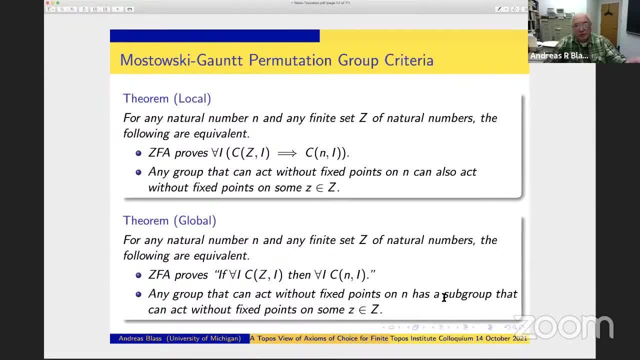 So the difference between the local and the global is that in the local group theoretic criterion the group itself that acts without fixed points on N should act without fixed points on something in Z, whereas in the global it's a subgroup that does the job. 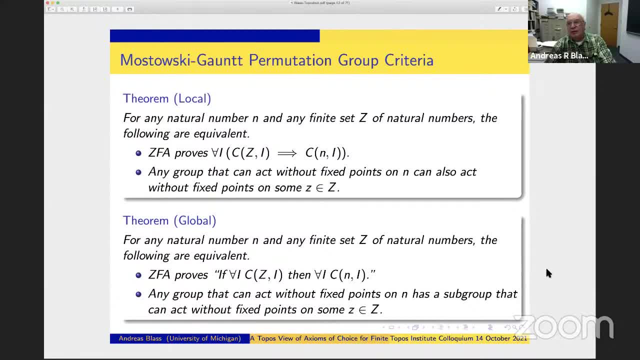 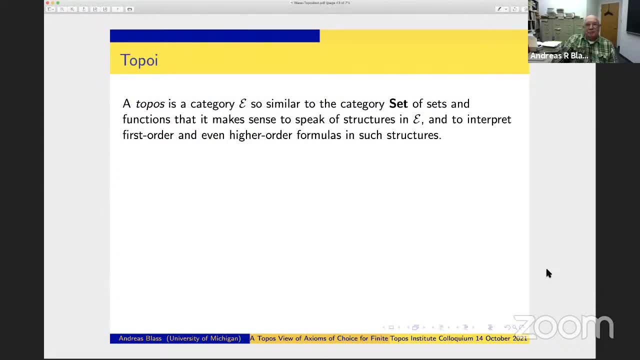 Okay, So those are the theorems of Mostovsky and Gaunt. I promised to say something about topoi in the topos colloquium, so I think that would be a good idea. Fortunately, I don't need much information about topoi. 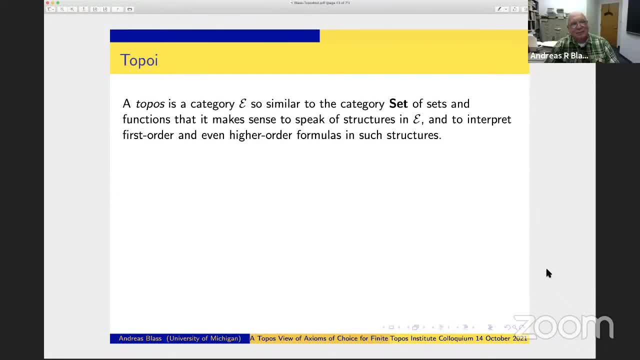 So I'm going to say some generalities. I'm not even going to define what they are. Sorry, can I ask a small question before you continue, please? So just on the previous slide I was wondering like: can you give? 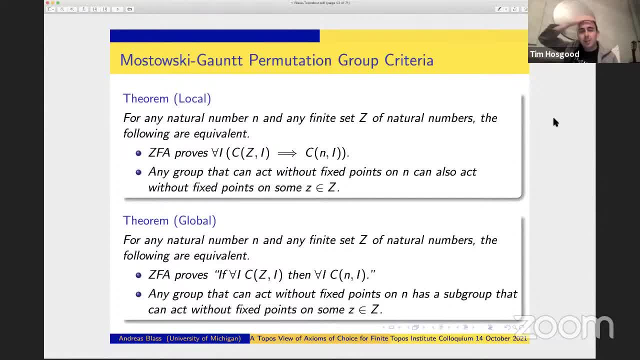 so you've already told us that, like the sorry, let me get this right- that the local statement for two and four isn't true. right, This is Yes. Can you give like an example of a group? Maybe it's obvious and I'm missing it. 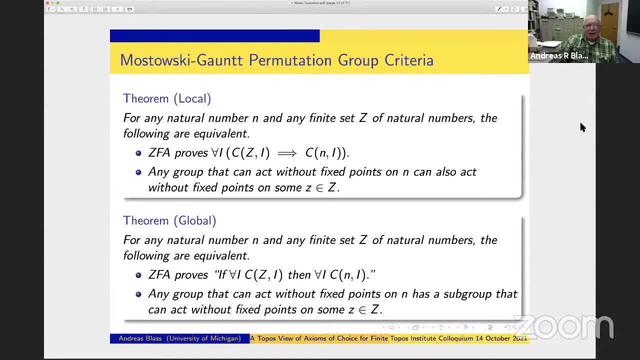 What is the group that like is the Entirely obvious. So I need to give you a group that can act without fixed points on a four element set, but cannot act without fixed points on a two element set. Okay, And I'm going to say the group. 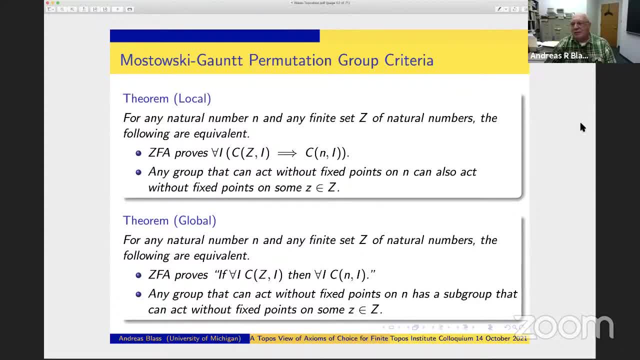 but the natural group that does this is the alternating group on four points. It acts in fact transitively on the four points, So fixed points. But the crucial thing is that it has no subgroup of index two. It's a group of order 12. 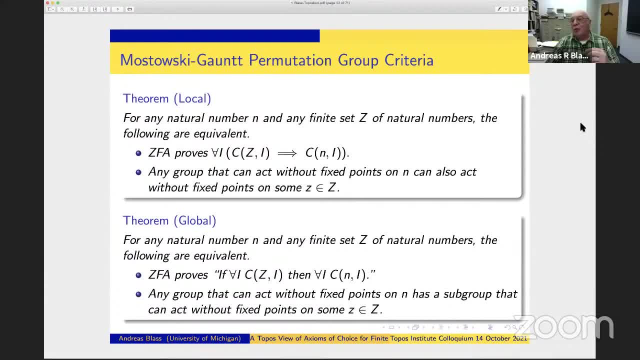 with no subgroup of order six, So it has no quotient of order two And if you're going to act on a two element set without fixed points you have to have, that's, a homomorphism onto the permutations of the two elements. 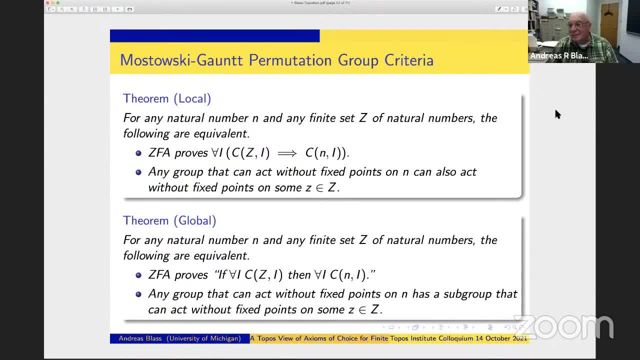 Okay, And just to finish that train of thought before I derail onto something else, the construction of the Franco-Mustafsky model, where choice holds from, say, countably many two element sets but not countably many four element sets, that Franco-Mustafsky model is built. 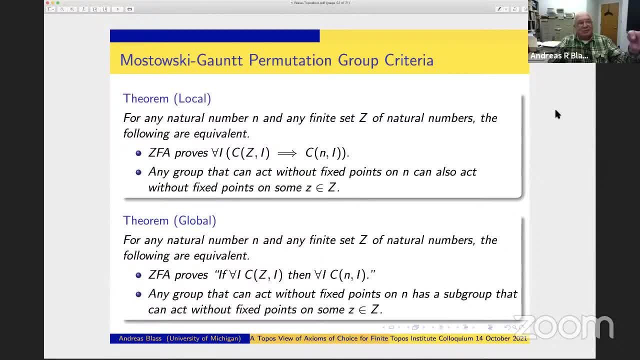 using a set of atoms- that is countable- union of some four element sets and a group of permutations that's essentially the direct product of the alternating groups in each of those four element sets. So the same group that goes into the second bullet item ends up being used also in the first bullet item. 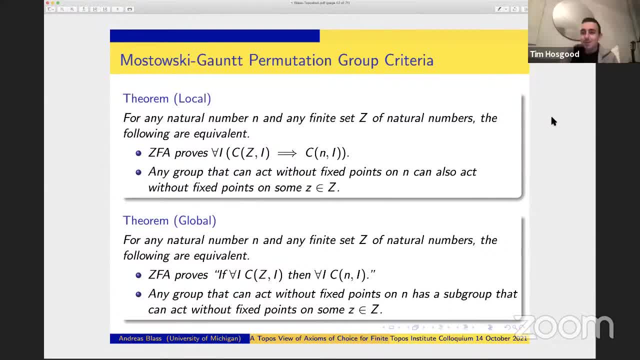 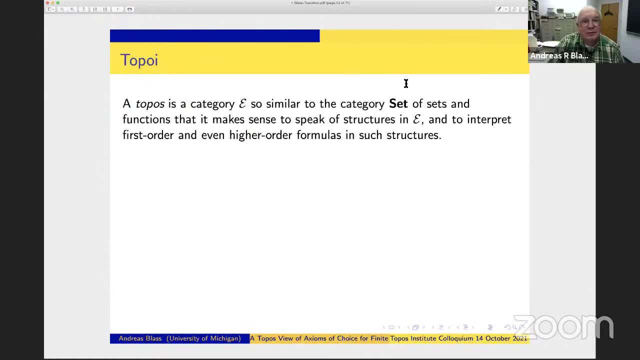 Just in a slight way, Thank you. Thank you, Okay. Okay, Now that I'm looking at chat, I see that there are questions there. Is there, Let me take a look. What's in chat? CFA- Must the subgroup be non-trivial? 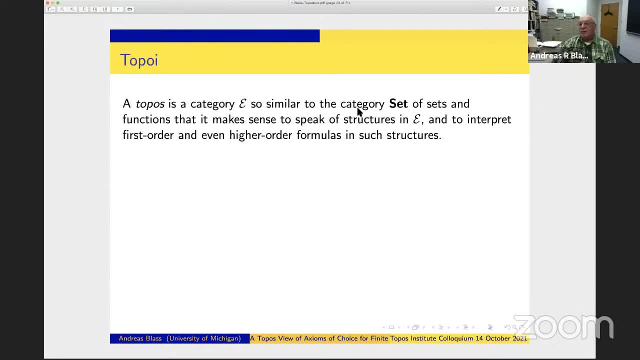 If you're going to act without fixed points on a set, then you have to be non-trivial, except for degenerate cases, right? When can a trivial group? A trivial group acts on a set by not moving anything, so everything is a fixed point. 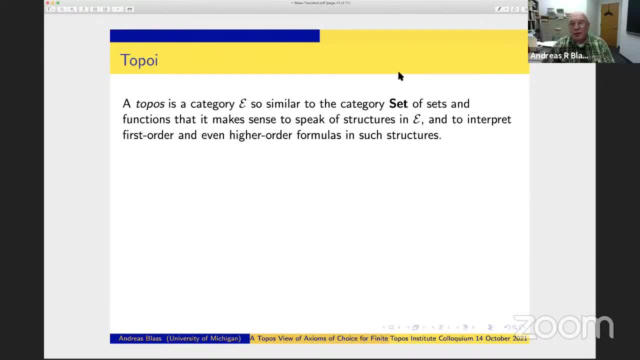 So if it's going to act without fixed points on a set, that set is going to be empty, And that's just as well, because we don't want n to be. We don't want to do choice from zero element sets, Nor do we want to do choice. 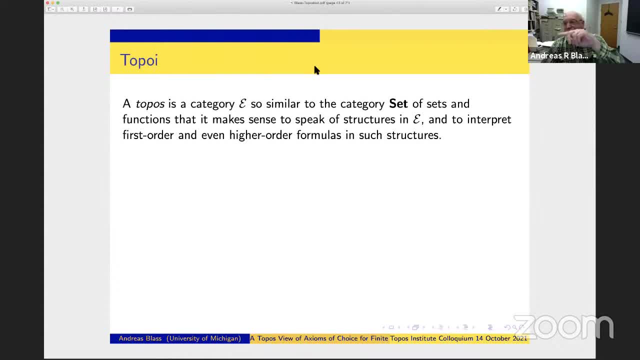 from one element sets. The former is always false, The latter is always true, So forget those. Yeah, Fixes every element. Okay, Yeah, All right, So I am out of chat again. What's a topos? So this is how we should think of a topos. 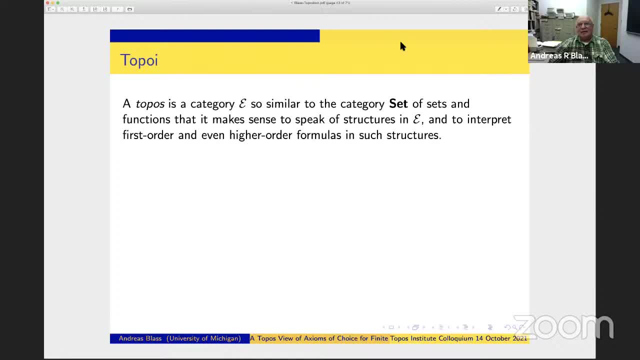 for the purpose of this talk. It's a category that's like the category of sets and functions And it lets you do most of the constructions that you do in ordinary set theory: Unions, power sets, Cartesian products, sets of functions. 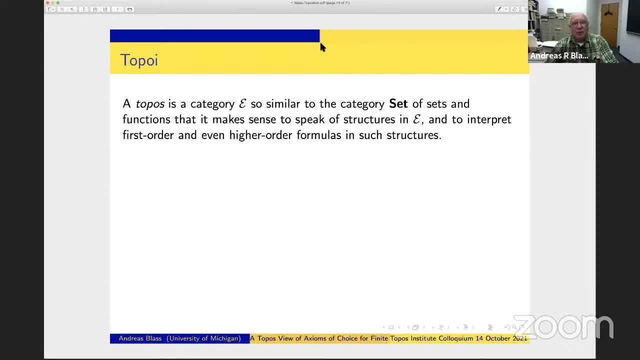 all kinds of stuff like that So similar that it makes sense to speak of structures- Structures in the usual sense of logic, a set with a bunch of relations and functions, All right- And to interpret first order and even higher order formulas in such structures. 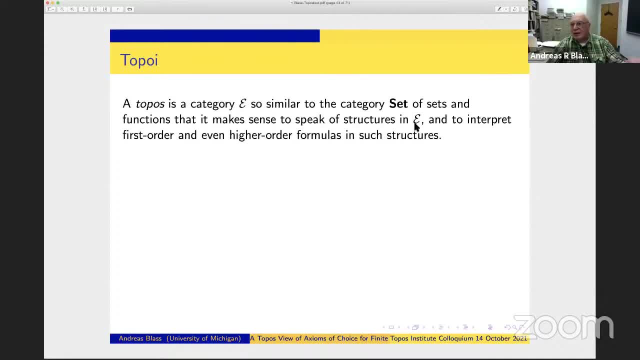 So, first order formulas: you want to know that you can interpret equality, interpret relations, holding of some elements, interpret functions of functions applied to elements For higher order. you want to have power sets and spaces of functions, and so on. A topos gives you all of that. 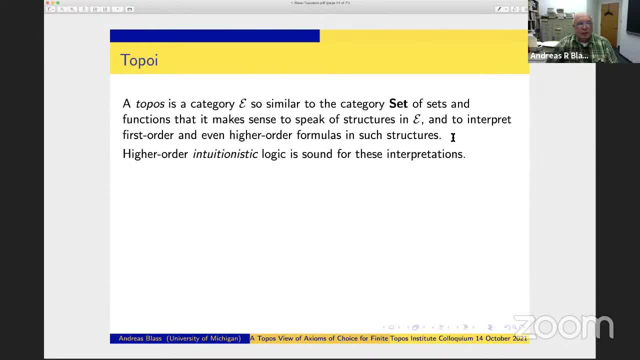 Okay, Higher order, intuitionistic logic is sound for these interpretations in any topos, In some topoi, but not all classical logic is sound. Those are called Boolean topoi in honor of George Boolean, People who invented classical logic. well, that's a mistake. 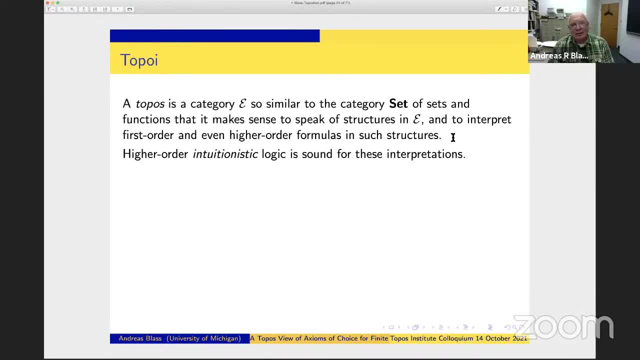 but I guess not. The most important topoi in this talk will in fact be Boolean, but the general theorems are going to be about arbitrary topoi. So higher order, intuitionistic logic, is sound. Did I want to say anything else? 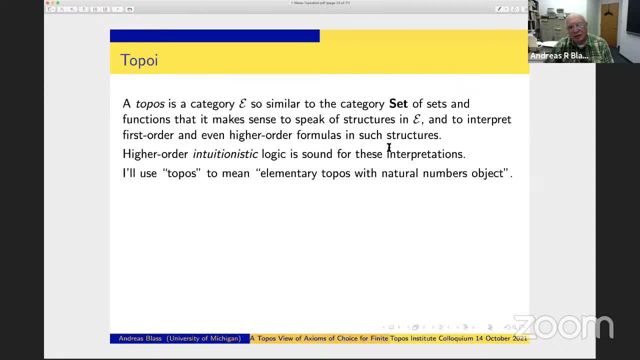 Oh yeah, I want to use topos. A topos can be an elementary topos. I don't need Grothendieck or anything like that, but I do want to have a natural number. object: I do want, I did want. 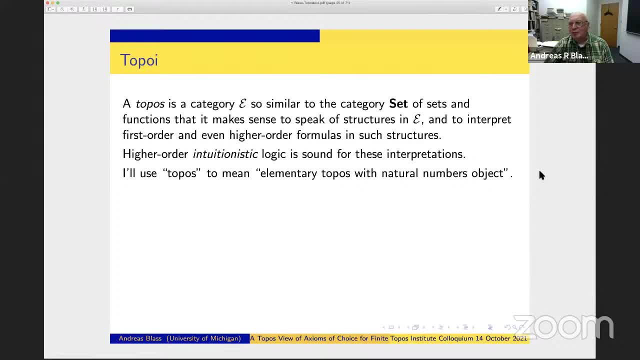 I'm not sure I really need it, but I've written out the proofs carefully. only in the case when there is a natural number object, I think they can be transported even when there isn't one. But just to cover myself in case I messed something up. 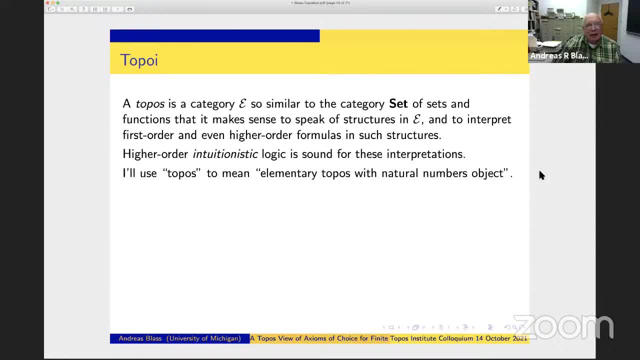 assume there's a assume, the axiom of infinity. Let me point out also that interpretations of sentences in this so-called internal logic, or the interpretation of sentences in a topos, may not look exactly like what one would sometimes think of, even in category, theoretic terms. 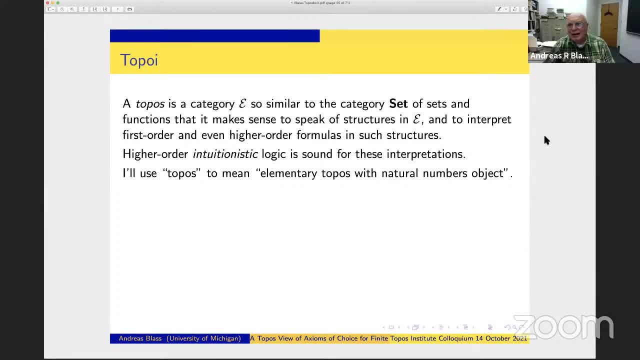 And maybe I will postpone saying any more about that until I get to some examples. So here's, here are some things about topoi. I'll start with the important examples for this talk. Well, I guess the first important example is the category of sets. 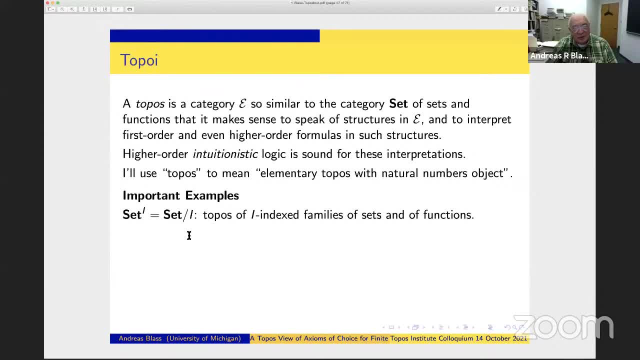 I'm doing set theory But there's a variant of that. Given any set i, I can form the topos of i-indexed families of sets which has two standard names, sets to the i. that's reasonable, An i-indexed family of sets. 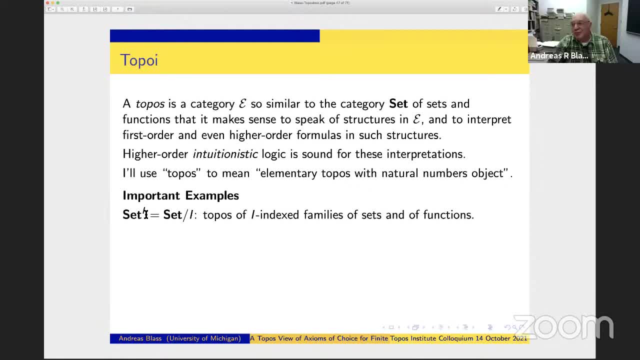 is a function from the index set i to sets. Another name, set slash i or set over i refers to a standard way of representing a family of sets within the universe of sets as a single object, not just as a function. You think of the index set. 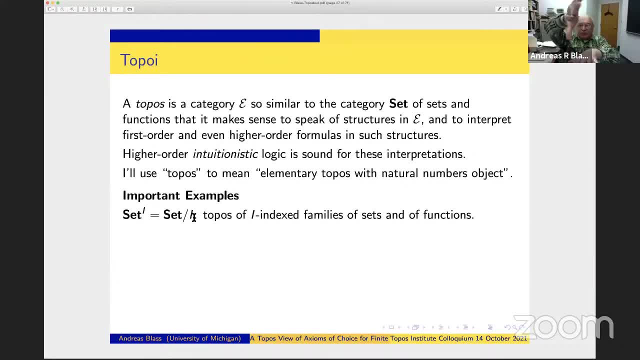 as laid out horizontally and stacked up over each index is the set that it indexes. So you're sort of thinking of this joint union of all the sets in the indexed family. This is a topos, Its whole structure, sort of works, index by index. 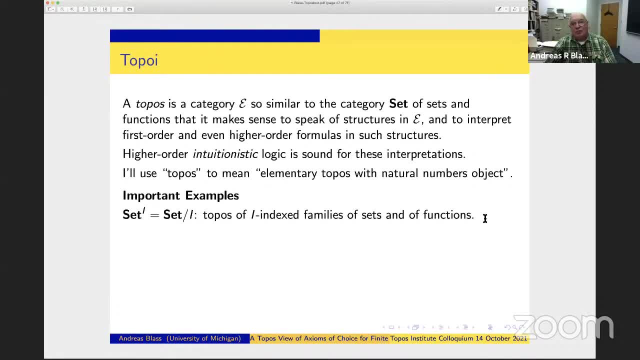 So a structure, let's say a group in this topos, would consist of an i-indexed family of groups And a statement about the groups, like say this group is a billion would be well might be true for some indices and false in others. 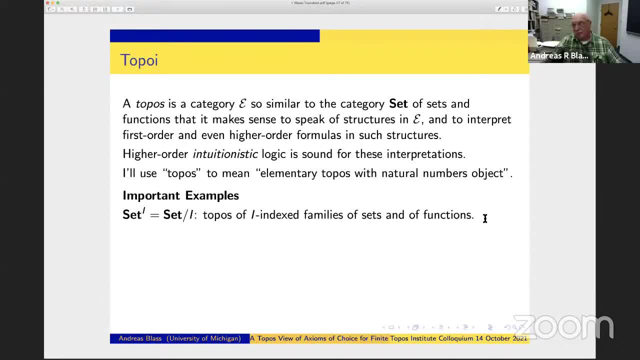 Its truth value would be the set of those indices where it's true. So the truth values in this topos are subsets of the index set. There are variants of this. You can take a model of ZF rather than the standard category of sets. 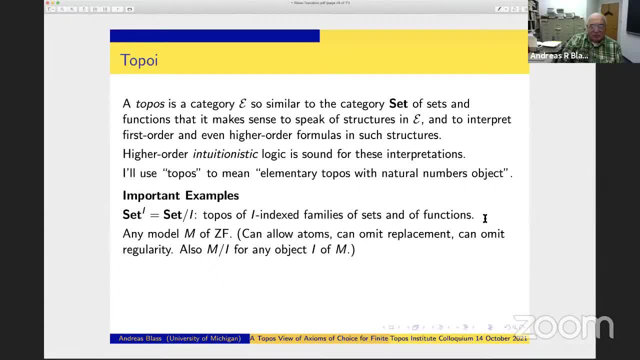 And it doesn't have to be real ZF. You can allow atoms, so you could use ZFA. You don't need the axiom of replacement, You don't need the axiom of regularity. So there's a good deal, a good deal. 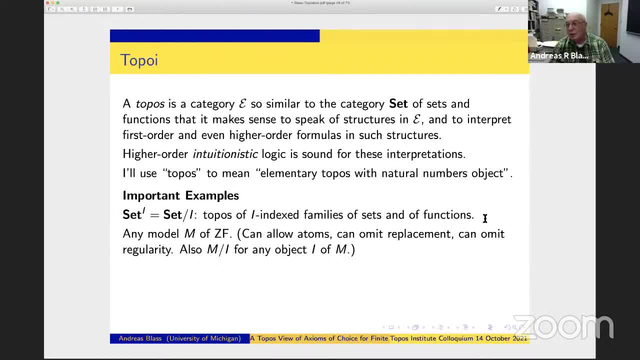 a model of a reasonable set theory is going to be a topos, And in fact a Boolean topos Also. you could do m over i for any object that would consist of the. an object in this so-called slice topos would be i and something with a map to i. 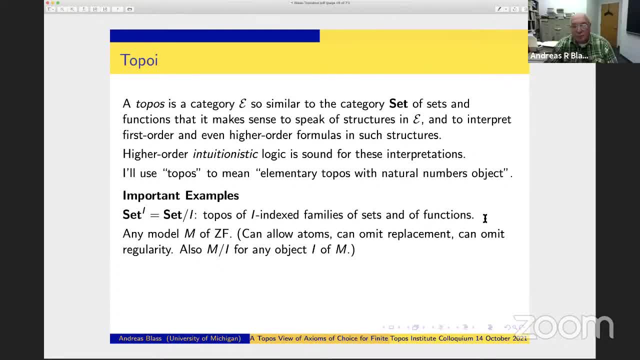 The idea being that the fibers of the map are supposed to represent the sets indexed by the elements of i. So this is one of the important examples, And we'll see in a minute why it's important. Another important example: Fix a group G. 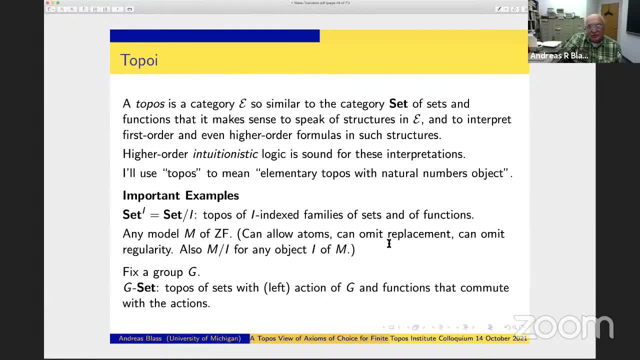 There is a topos whose objects are sets with a specified action of G. So the same set with different actions is a different object. The morphisms in this topos are functions that commute with the action. Okay, This is another nice example of a Boolean topos. 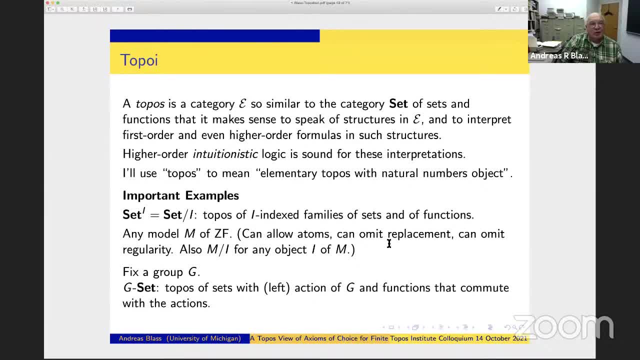 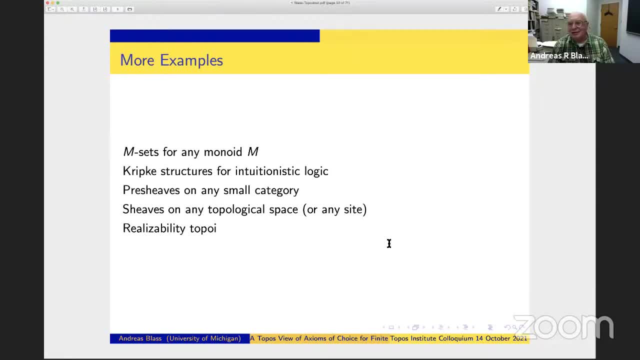 So these are the important examples. I think the next slide is unimportant example. I didn't say it that way. More examples, But this is just there to indicate that there are a lot of topoi around Instead of using a group in that last example. 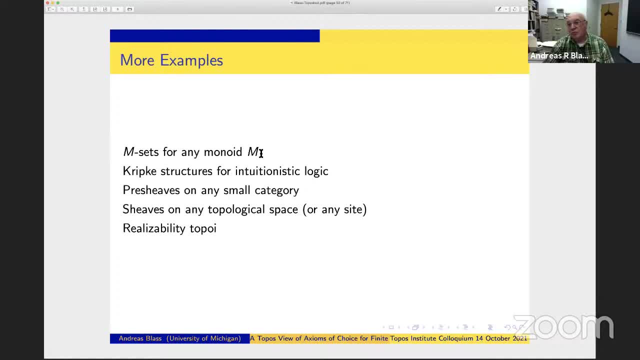 you could use a monoid. That would not be a Boolean topos anymore, unless the monoid happened to be a group. You can get intuitionistic logic: Kripke models constitute a topos, A generalization of that pre-sheaves. 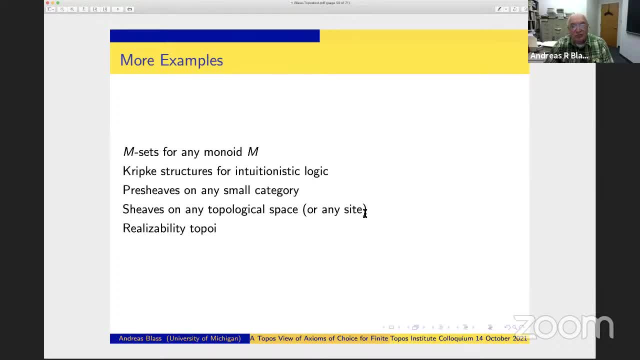 on a small category, A further generalization: sheaves on topological spaces or sites. There are realizability topoi For category theory. No, these are good for category theorists. For set theorists, here's one to chew on. Take some model of set theory. 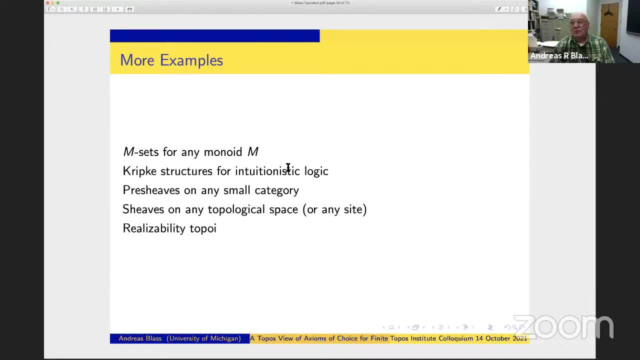 and look at the sub-universe of ordinal definable sets- And I did not say hereditarily ordinal definable, I mean ordinal definable. You can have an ordinal definable non-empty set that doesn't have any ordinal definable elements. 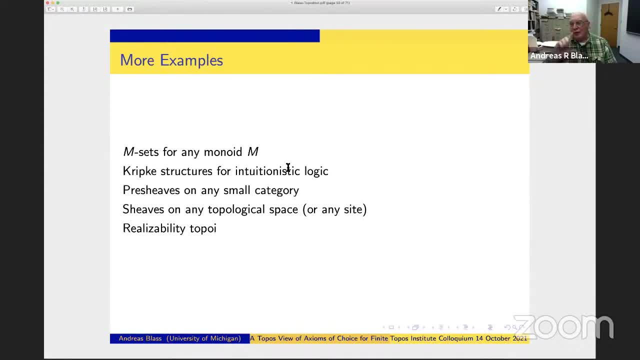 So in this topos it could be internally true, true in the internal logic, that this particular object has members, but it may not have any maps to it from one in the topos because there are no ordinal definable members. Strange things can happen between the internal logic. 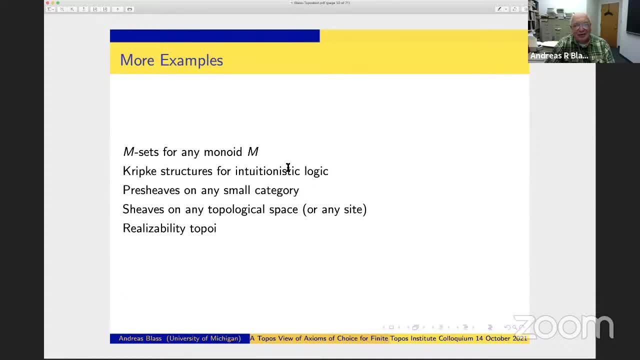 and what you see actually present in the category. Okay, back to the important examples. I want to say a little bit about these i-indexed families of sets. So this is a topos. my first important example: An object is an indexed family of sets. 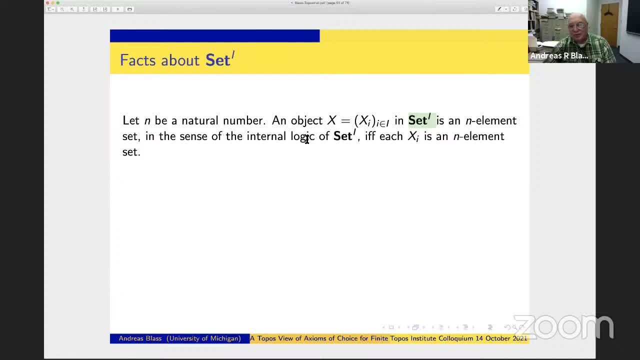 It is, in the internal sense, in the logic of that topos, an n-element set, just in case each of the sets in the family is an n-element set. It's about the simplest you could hope for A point. well, in general. 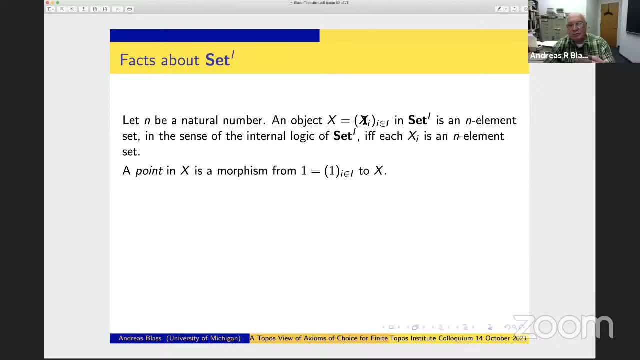 a point of an object in any topos is a morphism from the terminal object one into x. A point in this example is therefore, for each index, a map from standard, one element set into x sub i. That's a choice function. Points are choice functions. 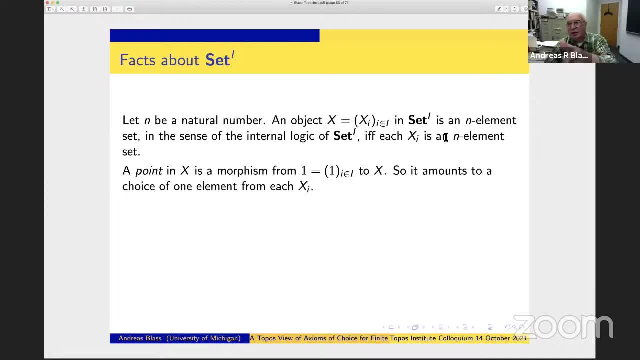 The internal logic didn't ask about choices. It just said each one individually is an n-element set. There's no guarantee that in general, without choice, that that implies the existence of a point, And that's the first crucial thing. Okay. 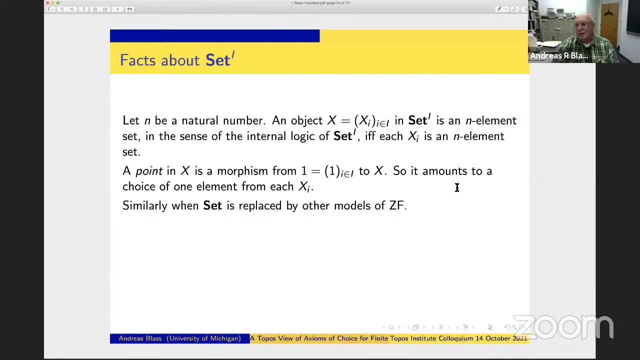 I'm going to gloss over that. Put other models of set theory in there, it still works. So to say, choice from i-indexed families of n-element sets is just to say that in this topos every n-element set in the sense of internal logic. 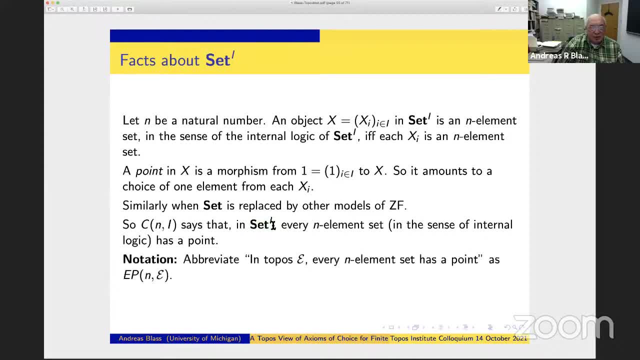 has a point. I think I have an abbreviation for that. Yes, To say that in this topos e, every n-element set in the sense of internal logic has a point. I'm going to abbreviate as ep for existence of points in n-element, objects in e. 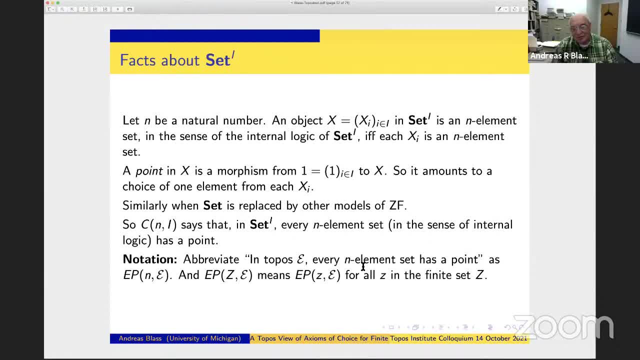 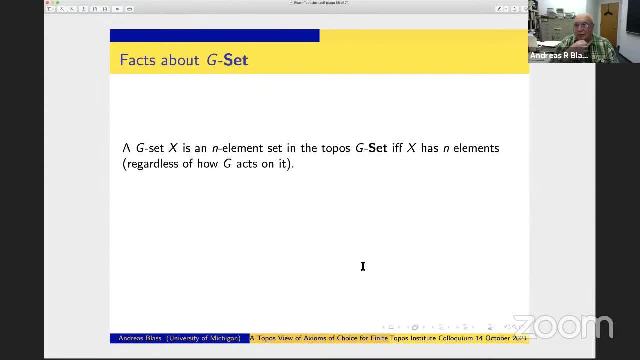 And same as before with the choice principles. if I put a z in there, a set of numbers, I mean for each of those numbers individually. Back to the second of the important examples: A, g-set. So we're looking at the topos of sets. 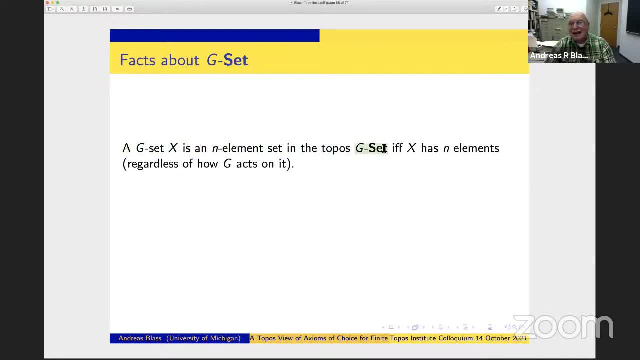 with a left action of g. Under what circumstances is that an n-element object in the sense of the internal logic? Well, you have to do a little computation and it turns out that it just means the set has n elements and don't care how the group acts. 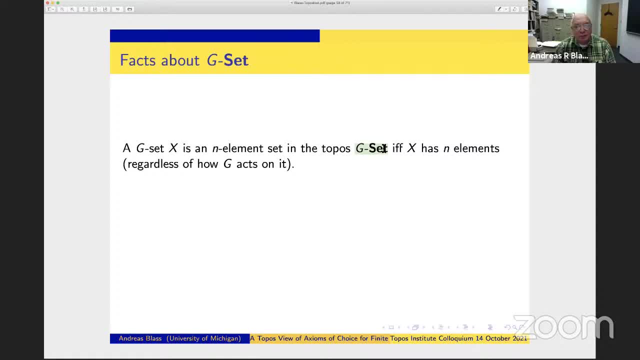 Again about as simple as you could hope for. A point, however, in a g-set is an element that's fixed by all the group elements. It's a fixed point of the group action. So my existence of points, principles for when interpreted in the sense of the topos g-set. 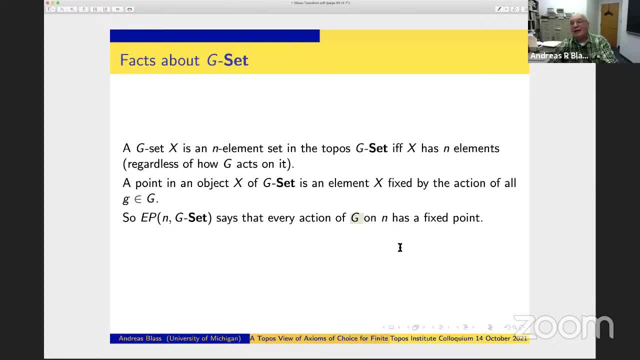 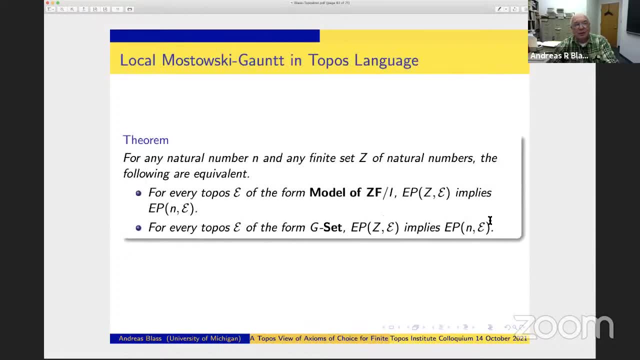 says every action of g on an n-element set has a fixed point, And the same with z in place of n. Big deal, Those observations on the previous slides. let me state the local version of the Mostovsky-Gonk results in the topos language. 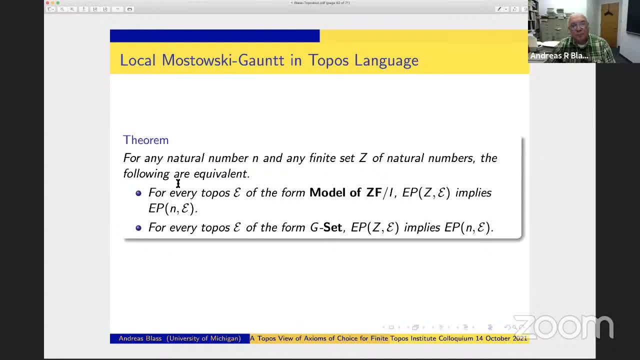 and they come out looking remarkably uniform. The choice principle says: if you take a topos of the form slice of a model of zf over an object, i, e, p, existence of points for z implies existence of points for n, And the group theoretic condition says: 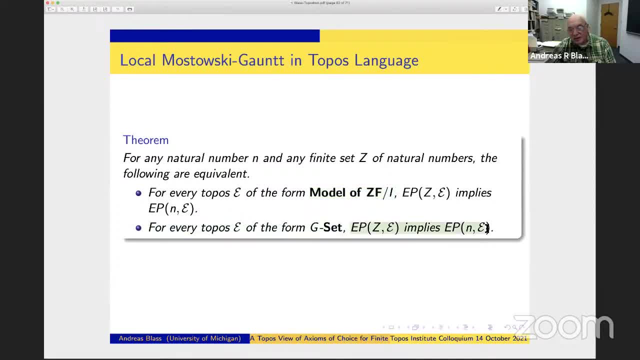 same implication: e p z, e implies e p n e. but now for topoi of the form g-set, The two equivalent conditions of Mostovsky and Gonk are topos, theoretically saying the same thing, but for two very different conditions. 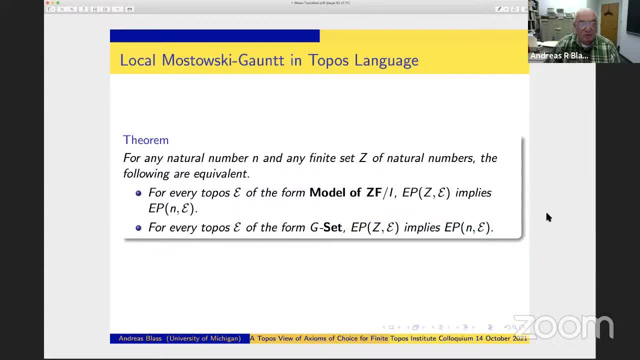 So it is reasonable to ask: well, is there anything like this? Are there equivalences for other classes of topoi? Is there anything like this going on? more generally, What other sorts of topoi does this apply to? Or maybe there are two other classes? 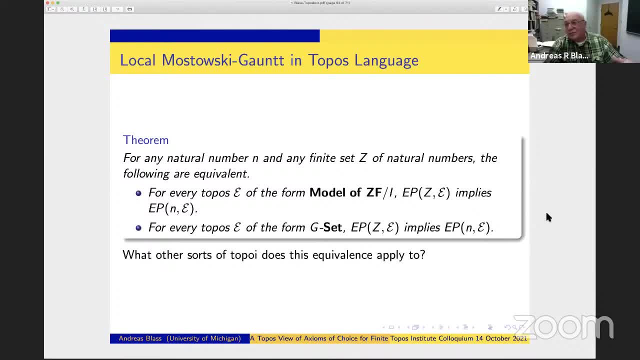 that are equivalent in the same way but not equivalent to these classes. You know what's going on And that's the first of the main theorems. since I have like two minutes, That's one minute per theorem. This is the general local theorem. 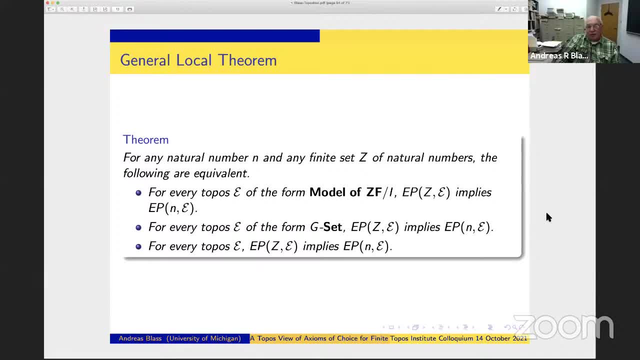 The first two bullet points are what was on the previous slide, And the third one is the new result. For every total, Take seven more minutes. Pardon, Okay, You have seven more minutes, yeah, Okay, All right, I'll talk slower. 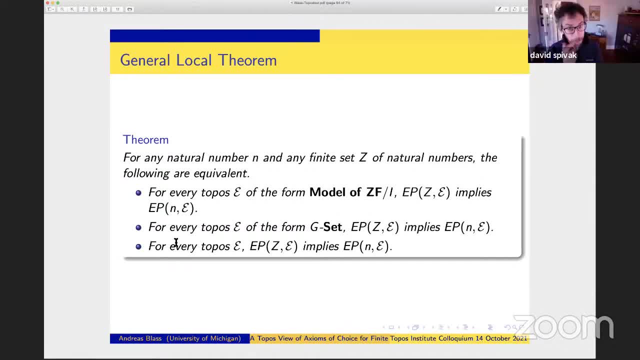 As you wish. The point is that for this to happen in slices of models of set theory and for this to happen in sets with a group action, if that happens, it's going to happen in absolutely every topos, not even necessarily Boolean. 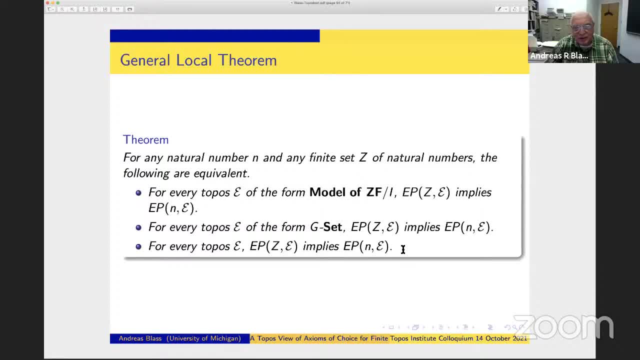 Monoid actions, sheaves, all kinds of stuff. Of course, one implication is trivial: If it happens in all topoi, then it happens in these examples. The essential part of the proof is to get from. Well, the way the proof works is: 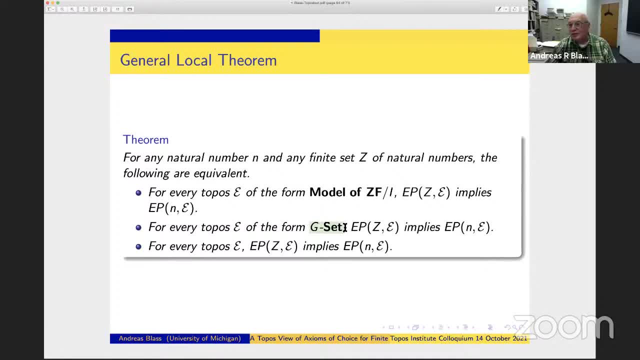 you start with the group fixed point, the Mostovsky-Gantt criterion in terms of groups, and you try to prove this in an arbitrary topos. The argument is similar to what was done in going from the group criterion to the choice functions principle by Mostovsky. 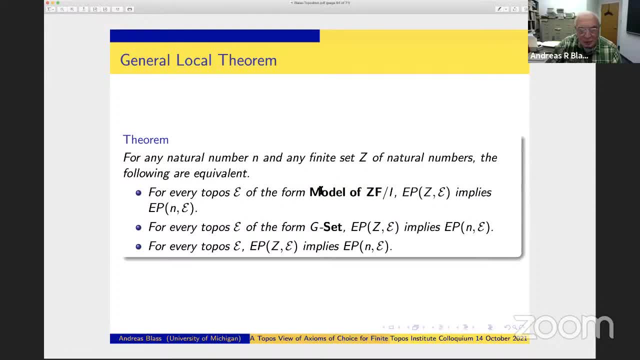 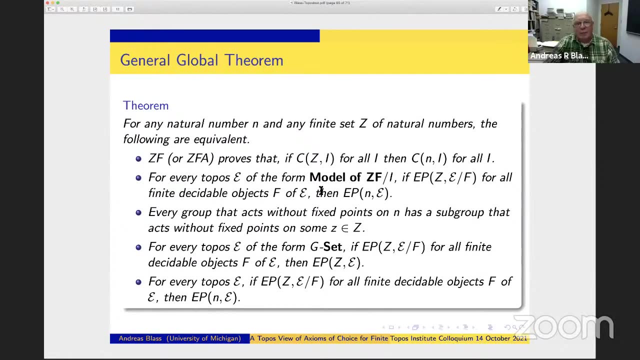 and later by Gantt. But of course it has to be adapted and manipulated a little, let's say to apply to arbitrary topoi The global theorem. Well, that's a long one, isn't it? So let me pick out. 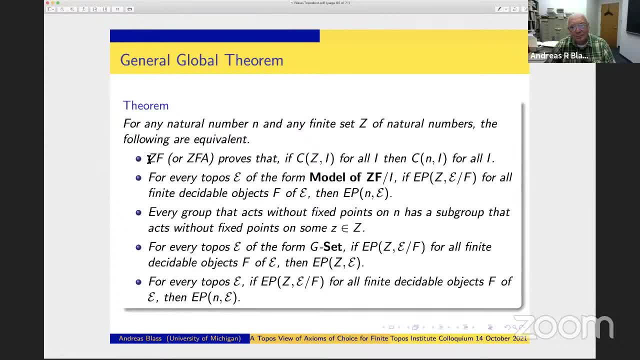 the important stuff. Bullet number one is global implication. The z-choice principle for all index sets implies the n-choice principle for all index sets. It's the global implication of the sort that Mostovsky was looking at originally. The second bullet is translating that into topos. 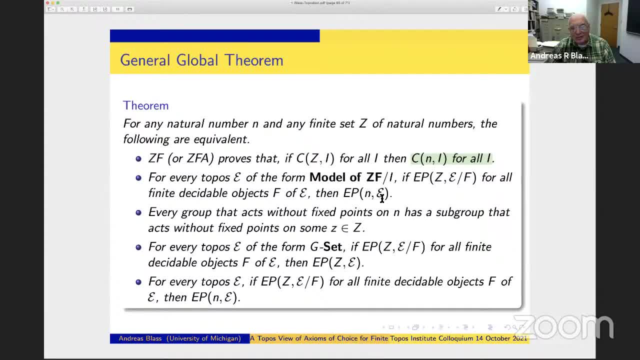 theoretic terms and the globalization shows up here That the assumption to get the conclusion about the topos E you need the assumption not only for E but for indexed families from E. you don't need very big indexed families. Indexed set can be a finite. 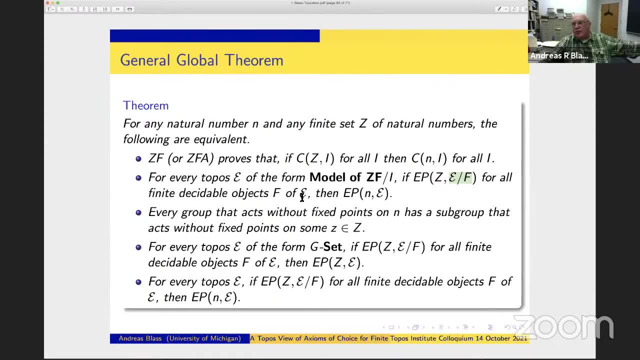 decidable object in E. but you do need something- This is like back in the original Tarski story- to prove something about countably many four element sets. you needed something for not so countably many two element sets but the not so countably many. 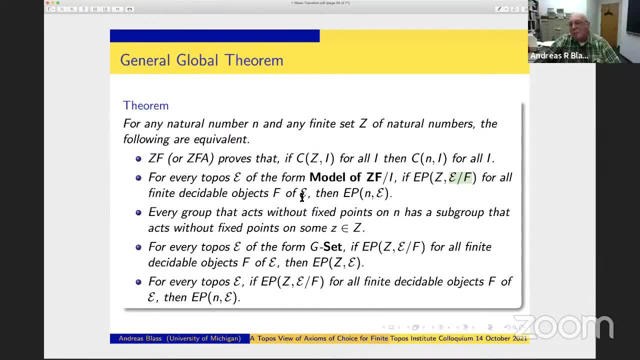 were only like six times more than the countably many. So the original family of four element sets. So it's that six to one family that's being abstracted here into this F Bullet. item two, three is the Mostovsky-Gantt criteria for global. 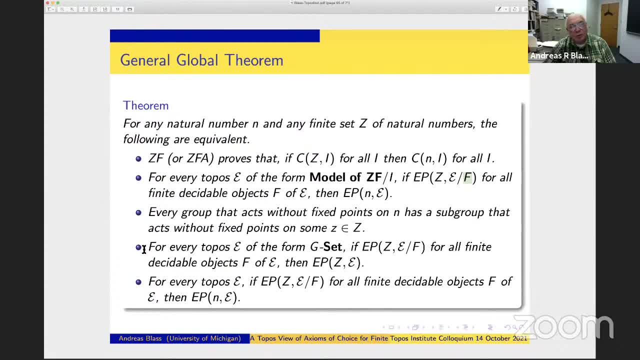 implications. Bullet item four is a topos theoretic translation of that into G sets and again differs from what we had in the local theorem by having here not just E itself but all its slices over finite decidable objects. And then the last bullet item. 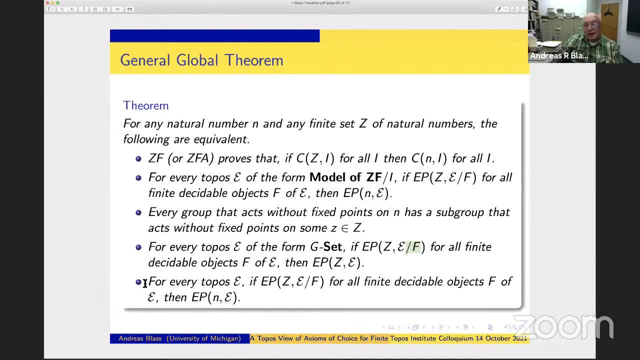 is not just observing results from before, but getting the new information that, just as in the local theorem, works for every topos. Okay, so those are the two theorems. I'm certainly not going to try, but I will say something. I think all that's left here. 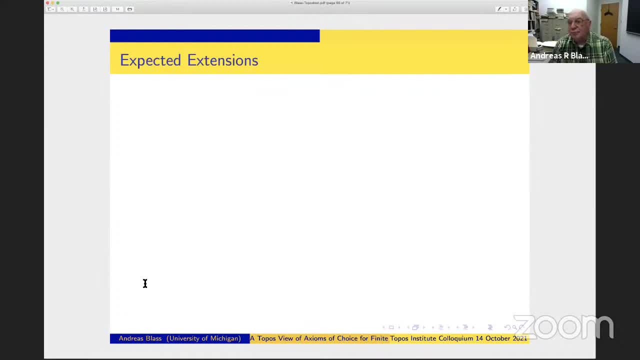 is about expected extensions. There should be more theorems. Let me describe what I think is going to be low hanging fruit, but I haven't actually plucked it off the tree yet. Choice principles: like before I put the choice principles, let me wave my hands. 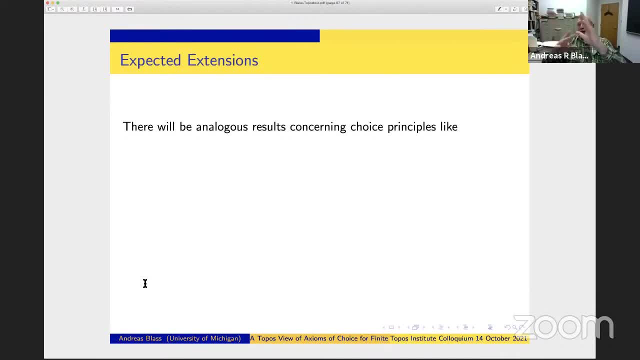 The choice principles. we've been talking about elements but no particular structure at all on them. We got a choice function which is putting a very particular structure, namely particular point. Oh, okay, I guess Paul has a question, but let me just finish one slide and then I'll shut up. 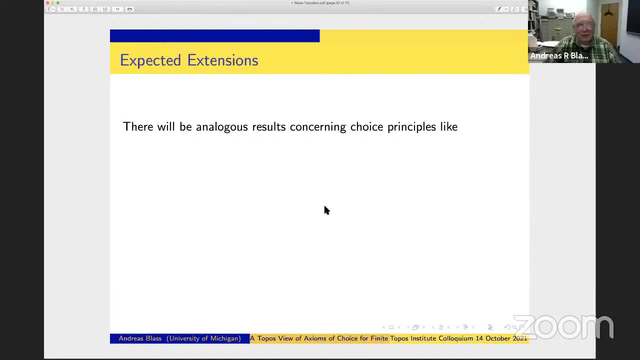 I was meant to ask you at the end. Okay, you're getting first in line. Okay, what I'm going to do now is work with- let me use the magic word- other species of structures, Instead of having something completely unstructured and trying to get a structure consisting of. 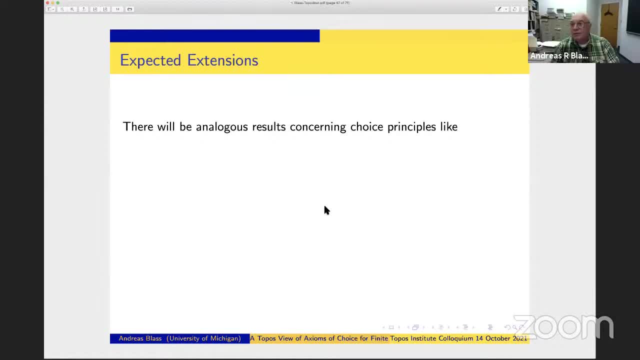 a single chosen point in it. you could do a lot of other things. Here's a random example. Given a family of seven element sets with specified orientations, any you know seven element set is a six simplex. it has two orientations. Suppose I pick one fruit. 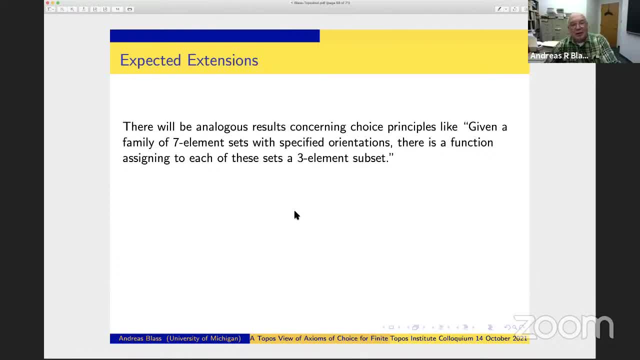 I'm given these seven element sets, but I'm also given an orientation. might there be a function picking for each of them a three element subset? So this is a randomly chosen example of a choice principle involving some structures other than the usual ones, In this case orientations. 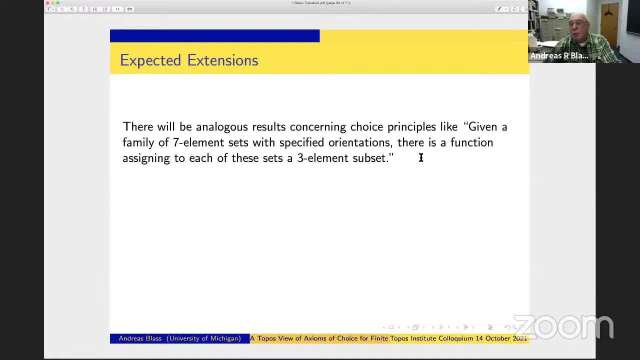 three element subsets. There should be group theoretic criteria that will concern groups that act on a seven element set, preserving an orientation but not preserving any three element subset. That's the analogue of acting on a set without any fixed points And the topos. 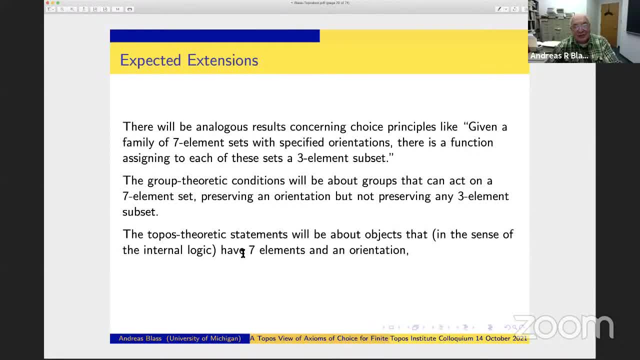 theoretic versions will be about objects which, in the sense of internal logic, have seven elements and an orientation, and then asking whether there is a point in the object of three element sub-objects, which I think is just asking: is there monomorphism from three into one? 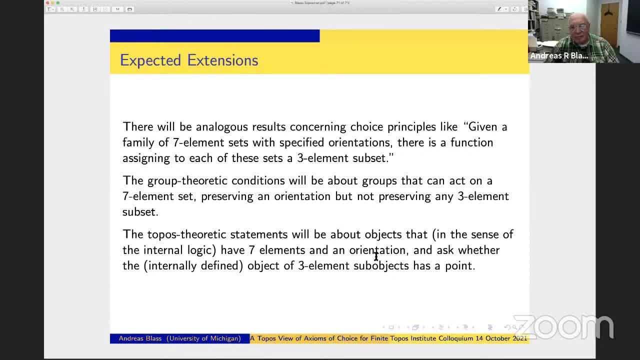 No, I take that back. That would be an orientation, A monomorphism from a family of three element sub-objects, three element objects. There should be equivalences for the set theoretic and group theoretic things. I believe this is already. 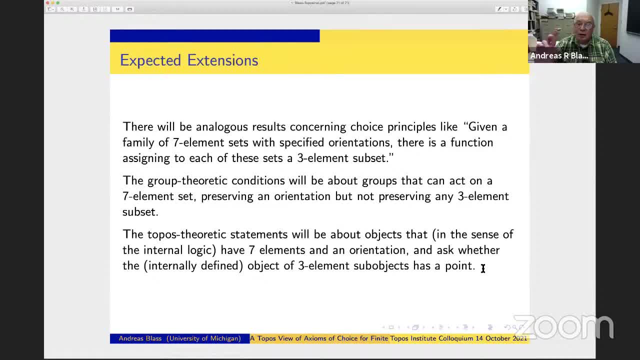 in John Truss's paper from 1973 and I am reasonably convinced that it should be straight forward to generalize that to arbitrary topoi. Okay, And I think that is exactly where I should stop. So I know Paul has a question and I see Let's first thank. 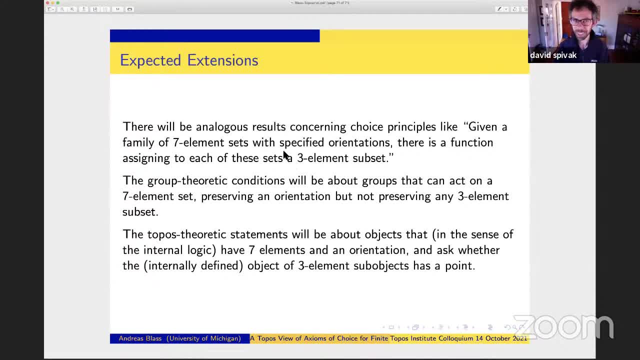 Andreas, so everyone can unmute or just clap in the emojis. Paul, would you like to ask a question? It's not often I say to a set theorist: that's a lovely talk. That was a lovely talk, Thank you. So I was thinking. 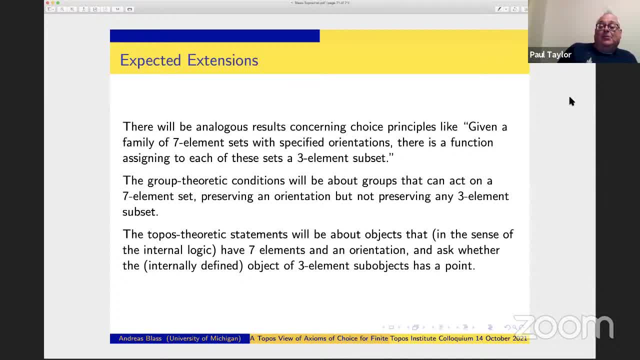 so my The natural example of where you would not accept choice would be something like choosing square roots on the unit circle of the complex plane: Correct, Right. So in other words, I'm thinking, Being more technical, I'm generalizing your results. 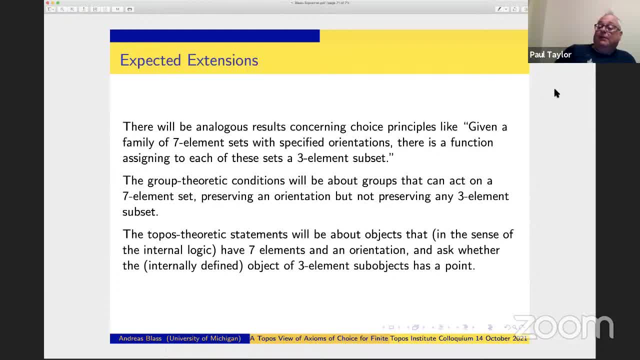 to sheaves over some geometric. I wonder whether the arguments continue to work and perhaps you could even put a number theoretic interpretation on the theorem. This is, I'm not sure we can get a number theoretic interpretation, but the results should, Unless I made a mistake. 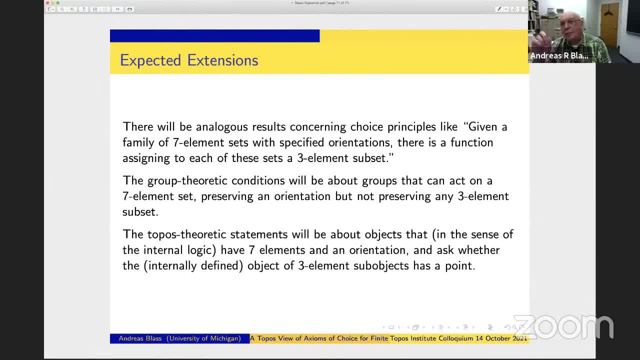 the results. I should make a comment on that, But that can come later. So let's see If you take, Let's pick square roots of points on. So we're going to take the unit circle on the complex plane and we would like to pick a square root. 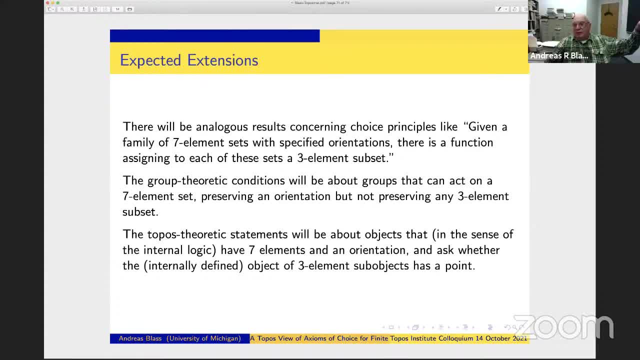 for each one, but when we do that continuously, we find ourselves at the antipodes. Okay, So that means What does that mean in sheaf terms? It means that we've got a circle, something which, in that sheaf, topos in the internal logic. 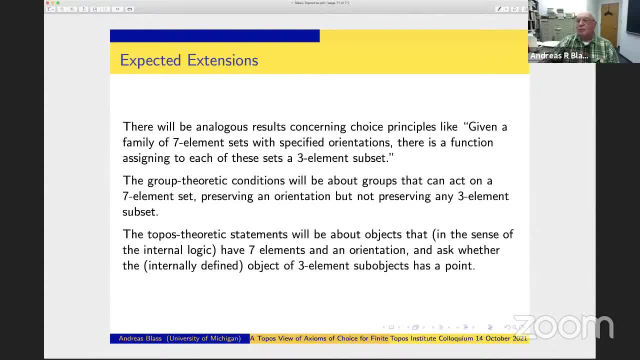 has two elements. It is internally isomorphic to the set 0, 1.. But it has no point. There's no continuous map from 1, which is the circle, to 2, which is this doubly wound circle. So what I called 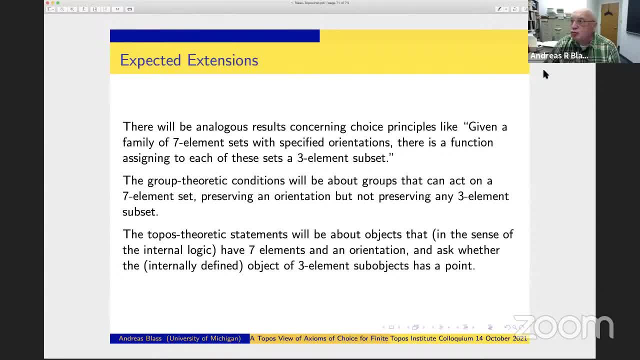 EP 2- Yeah, EP 2 for the topos of sheaves over the circle fails. Now Tarski will come along and say if it held, then we could also do choice from 4 in that sense. But We have to. 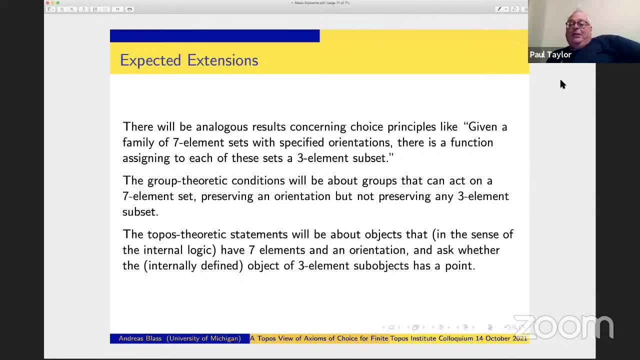 work a bit to think of geometrical interpretations of the choice principle. Geometrical interpretations are going to be things where, Let me see, Let me go out on a limb here because I haven't thought about this, But it seems to me that what would be important 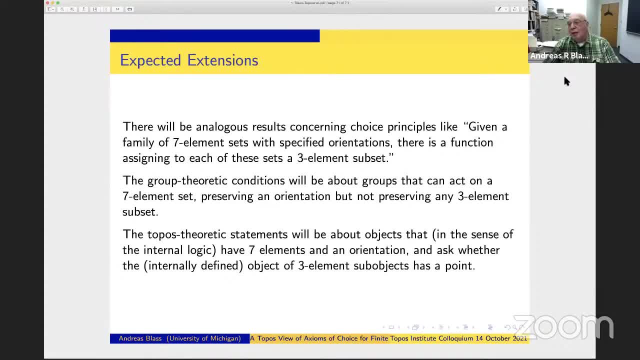 in cases like this, At least the following would be important. Maybe other things too, But what would be important would be things about the fundamental group of the space that you're taking sheaves over, Because choice principles like this- See what's happening here- is. 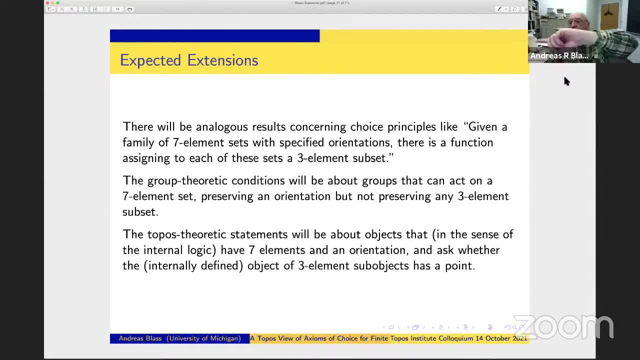 the fundamental group of that circle has a quotient of order 2 and that's why there's a two-fold covering And what one would want- I guess a better way to say it- is that quote: that fundamental group acts on a two-element set, without fixed points. 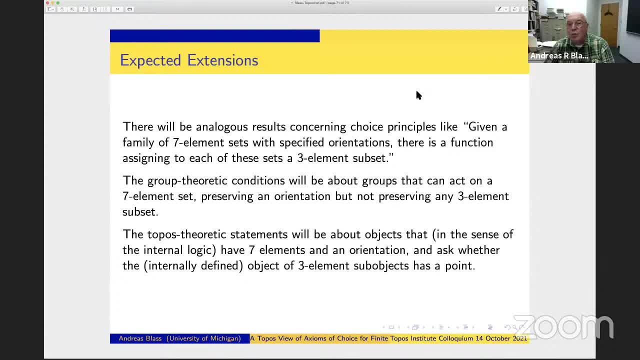 And I would expect that the one relevant thing for merging sheaf pictures with you know their toe point. My results apply allegedly to them, But to see the connection, I think one will end up with having at least the fundamental groups of those spaces. 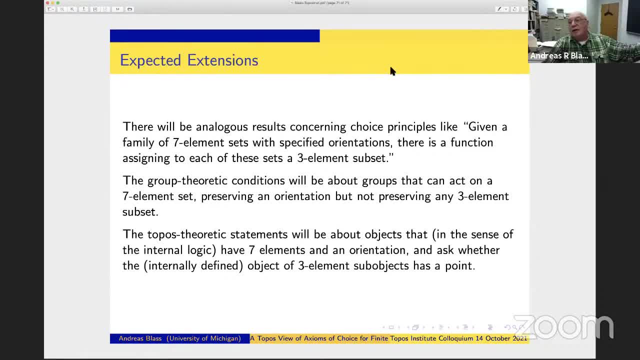 connecting with the groups in the Mostovsky-Gantt characterizations and probably also with the groups involved in building the Franco-Mostovsky models. So I claim without any solid evidence, without having thought about it very much, that there should be a connection between 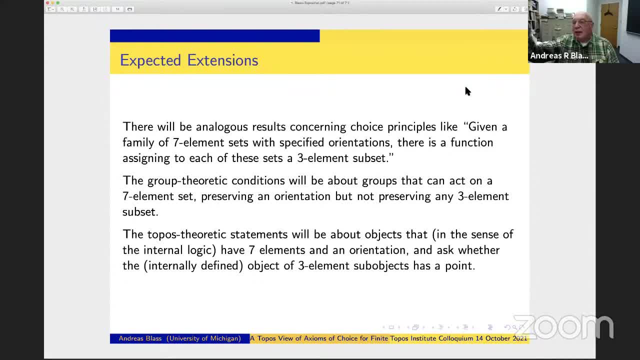 all the group theoretic things I ever mentioned in this talk and the fundamental groups of the spaces over which you want to take sheaves, And I think this fits reasonably well with ideas of fundamental groups being essentially defined in terms of covering spaces rather than in terms of 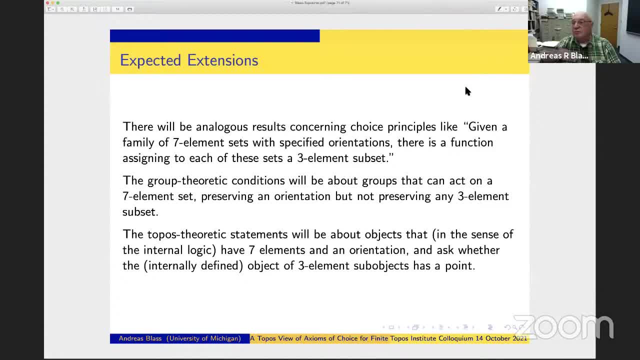 loops in the space and so on, Because here we're dealing with coverings, with sheaves over this thing and so on. So okay, I should. I've talked enough about what I don't know. You claim that your results were general. 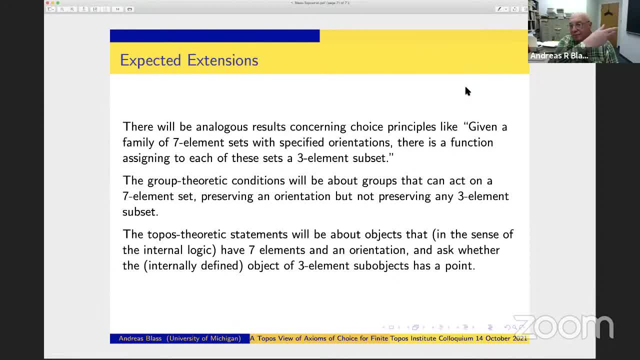 My results if correct. you know, they say for all topoi, that includes the topos of sheaves over the circle. yeah, Yeah, okay. Let me digress for a moment As to whether these results are correct So far, I have followed the. 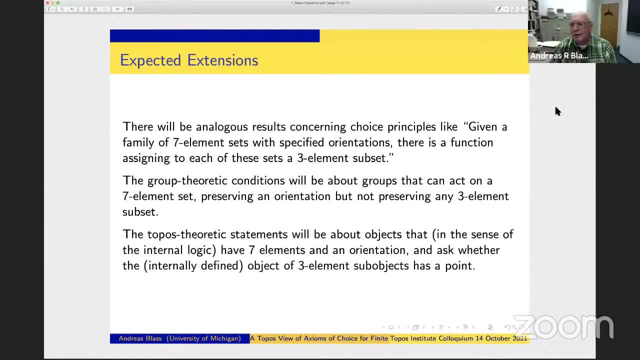 great tradition of Tarski and Gaunt in that, although I first talked about these results at a conference almost two years ago, I haven't yet written up the paper. And I've got a few pages done, but not much. So Tarski didn't publish. 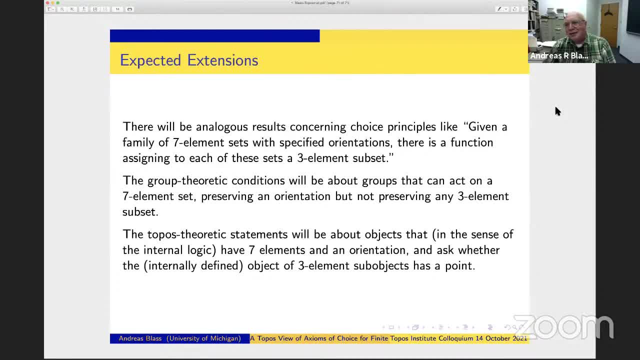 his stuff. Gaunt didn't publish his stuff and there's some danger here of continuation of the tradition. This last slide is my current excuse for not having things written up, because I think there are some extensions that should be fairly easily proofed by the same methods.